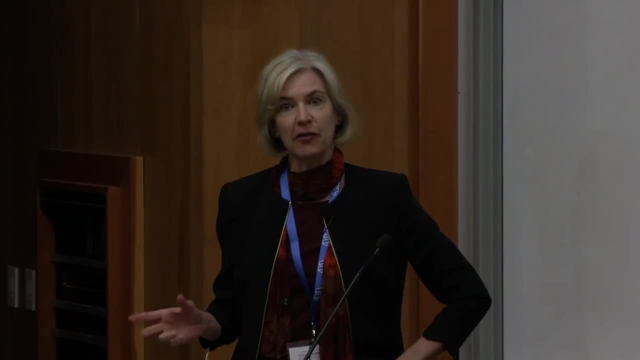 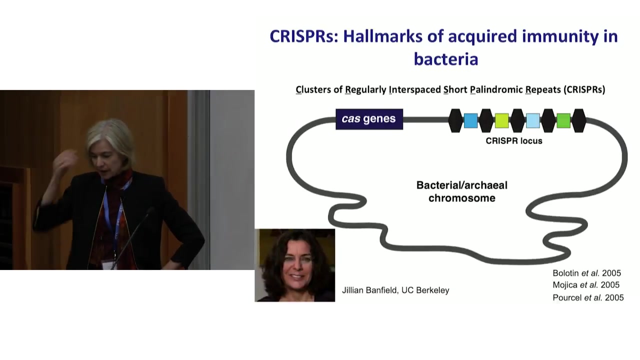 a very different purpose. So I'm going to talk about that And then I'm going to say a little bit about where I think this is all going. So the CRISPR field is a very young field. It's only really been around since the mid-2000s, when scientists discovered that a lot of bacteria have repetitive 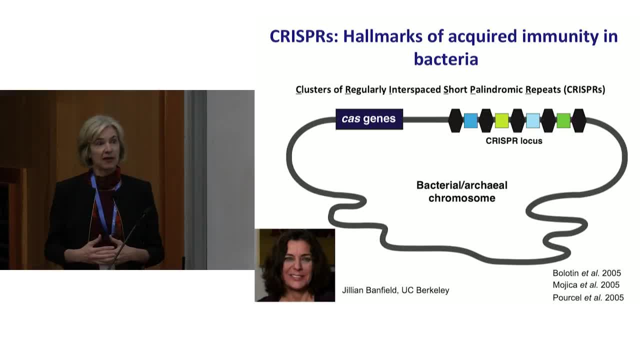 DNA sequences in their genomes. that came to be called CRISPRs, an acronym that stands for clusters of regularly interspaced, short palindromic repeats. A big mouthful. What does that mean? Well, it just means that many bacteria have a distinctive feature in: 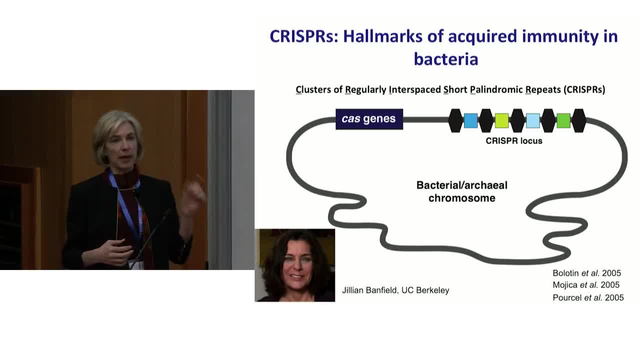 the chromosome, sometimes more than one, that include repetitive sequences shown by the black diamonds in this cartoon that flank unique sequences shown by the colored boxes, And three research teams in the mid-2000s noticed that in many cases there was no. 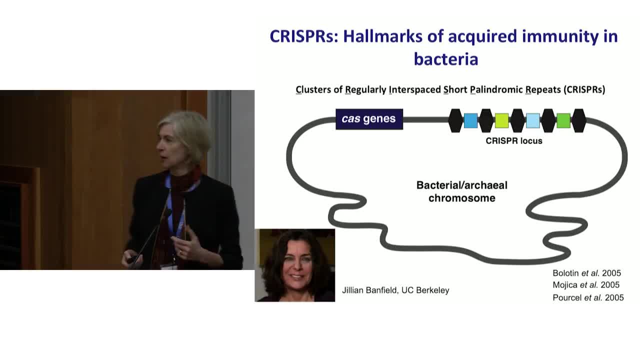 such thing. So what they found is these unique sequences in the CRISPR arrays come from DNA found in viruses. So this was the first indication that these might in fact be some kind of acquired immune system in bacteria. And scientists also noticed that, together with these arrays, 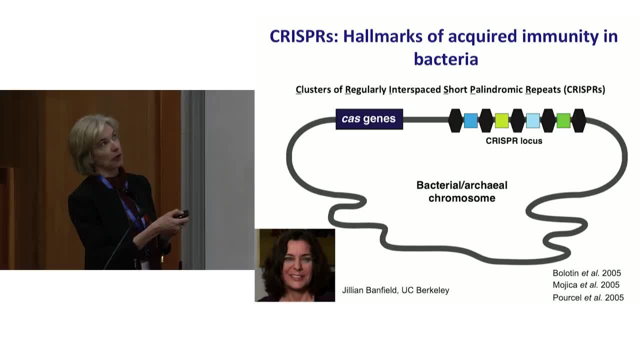 were CRISPR-associated or cast genes, typically located nearby in the bacterial chromosome that turned out to be encoding proteins that are part of this adaptive immune system. So this is the first indication that there was some kind of acquired immune system And our 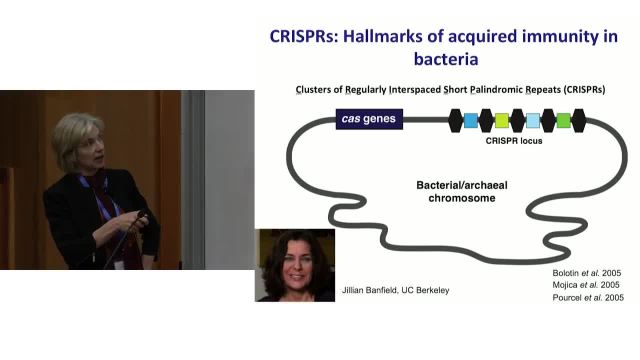 own research at Berkeley started because of the work of Jillian Banfield, a scientist here at Berkeley who does research on bacteria, typically on uncultured, unidentified bacteria, And her research uncovered the fact that many bacteria that you can isolate in various environmental 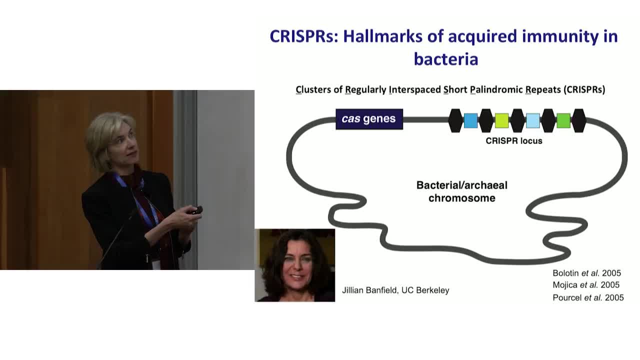 niches are very abundant in these elements, And so they are probably very actively using this kind of immune system to protect themselves from viruses in the wild. So it's some very interesting biology, And so I'm going to show you a very short video that illustrates. 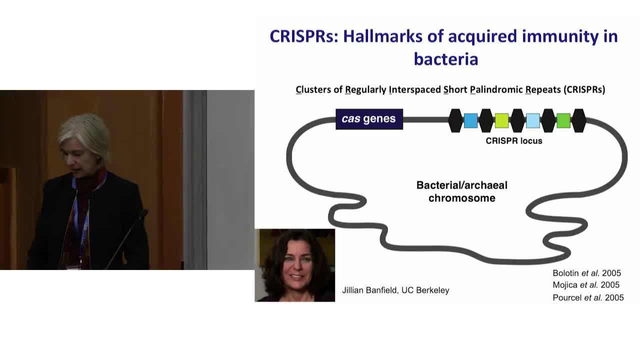 how these actually function and how the activities native to these bacterial immune systems are very, very nicely relevant to the work that Dana just talked about, because what they do is they make targeted cuts in DNA. So in bacteria this is happening to protect cells from viruses. but we can, as you heard, 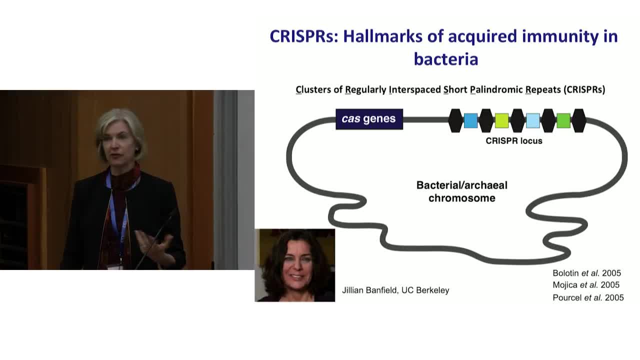 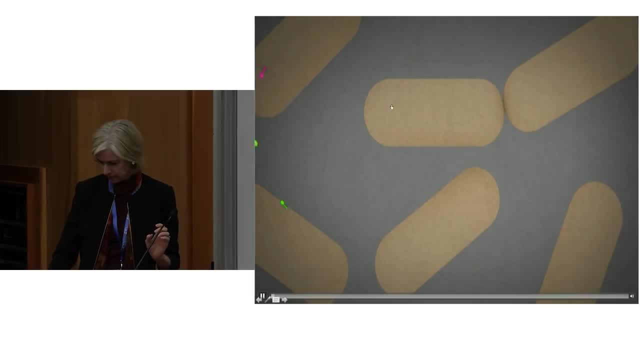 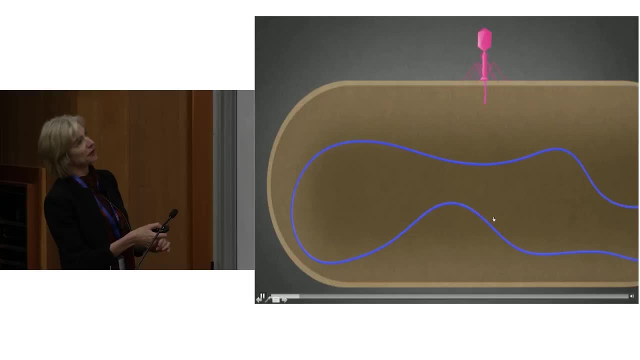 very nicely from Dana. this can be harnessed in various kinds of cells for gene editing. So I think my let's see if the audio works here. It's not okay, Well, I'll narrate this. So we have viruses that are entering a cell. You can see a virus injecting its DNA into. 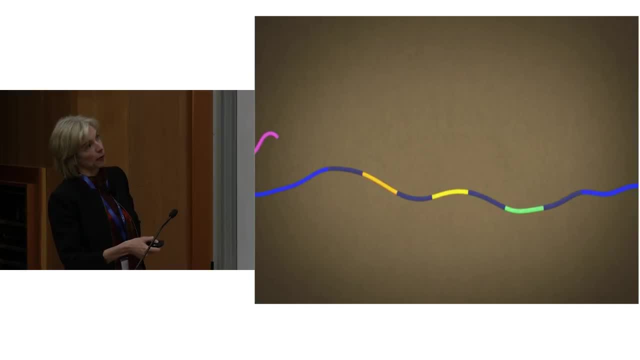 a bacterium. And if this bacterium has a virus, it's going to inject its DNA into a bacterium. And if this bacterium has a virus, it's going to inject its DNA into a bacterium. If this bacterium has a virus, it's going to inject its DNA into a bacterium. And if this bacterium has a virus, it's going to inject its DNA into a bacterium. And if this bacterium has a virus, it's going to inject its DNA into a bacterium. Now, as the cell is in the CRISPR array in the genome, it can acquire new pieces of DNA. 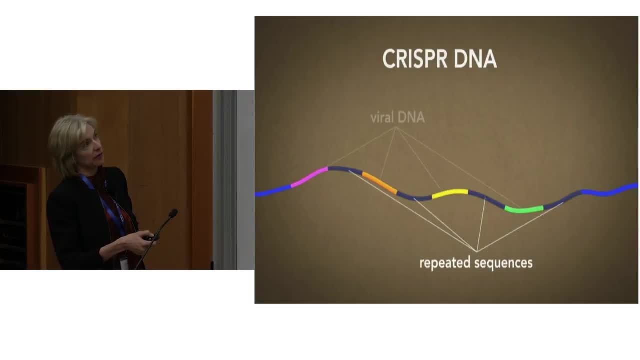 from the virus and integrate them into the array keeping this pattern of repeats, And the cell is then able to make a copy of that sequence in the form of an RNA molecule that gets subsequently broken into smaller units that each include one of the sequences derived. 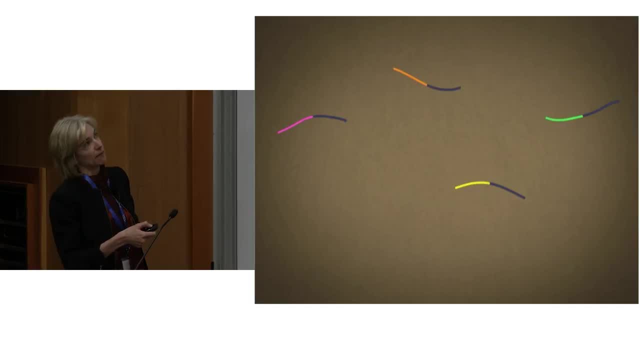 from a virus, together with the sequence coming from the repeat, And those RNAs are then kind of marked as CRISPR, as CRISPR molecules, by the presence of this repeat, and they combine with a second RNA called tracer to form a structure that binds to the protein called Cas9.. 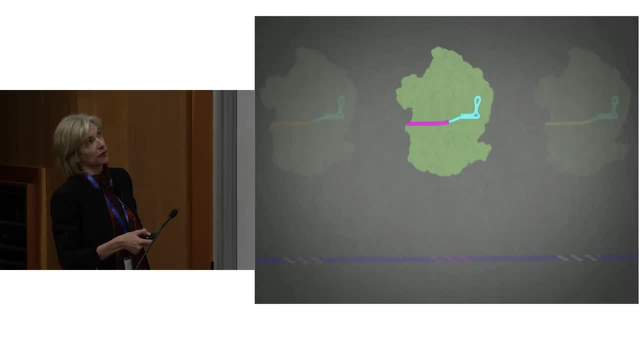 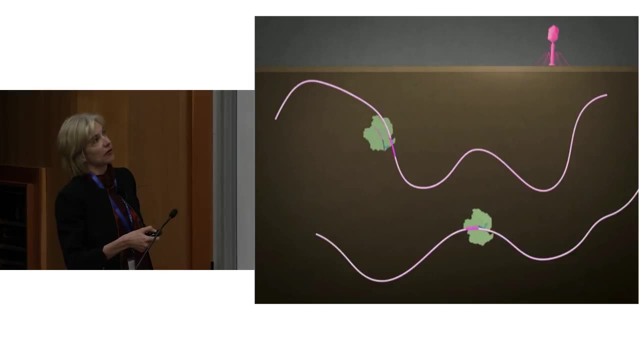 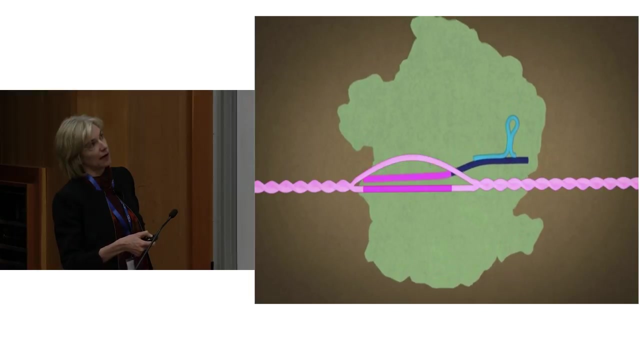 So this RNA protein complex then is able to survey the cell, looking for DNA sequences that have a sequence matching the sequence of the RNA, And if that match is found, then this protein RNA complex unwinds the DNA locally to allow RNA-DNA hybridization to occur. 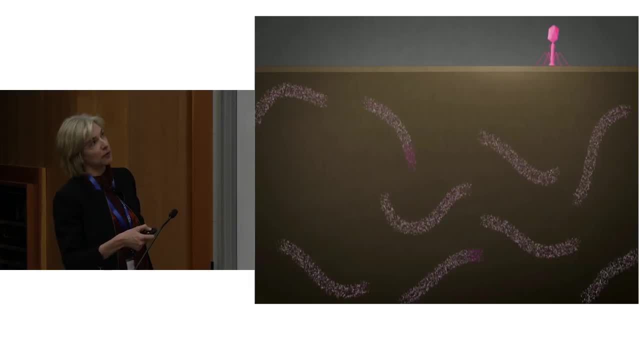 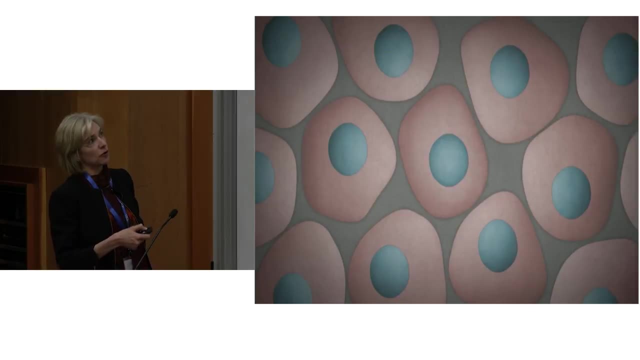 A double-stranded break is induced in the DNA and if this happens in a bacterium, that leads to degradation of the viral DNA. But if you introduce that system into a eukaryotic cell, a plant or an animal cell, as you heard from Dana, 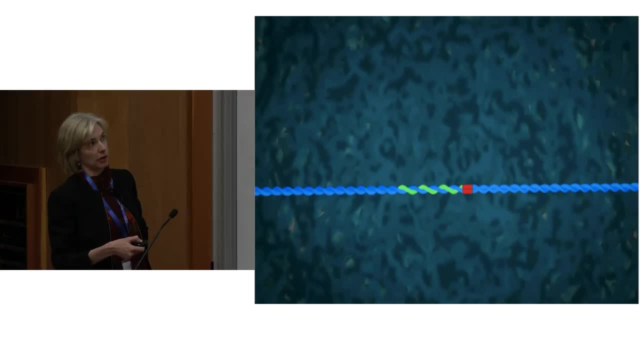 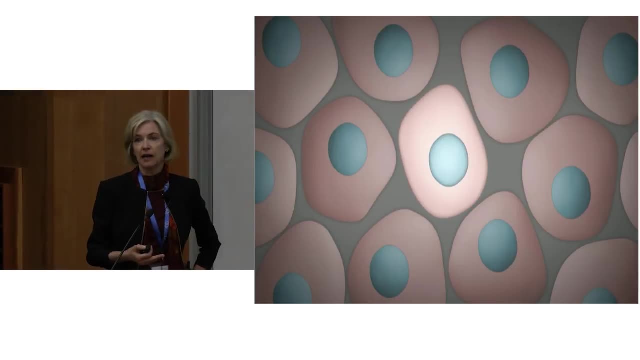 these cells have sophisticated machinery to repair double-stranded breaks, And they can do so by introducing a small change at the site of the break, or even by integrating a new piece of DNA during the process, And so that means that this method of introducing double-stranded breaks 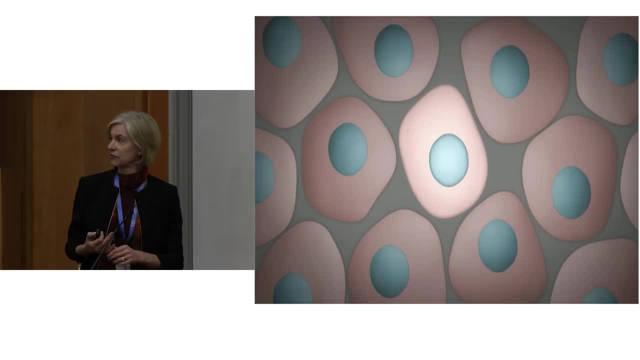 in a targeted fashion into the genomes of plants and animals is a very effective way to conduct genome engineering. So that's a very fast sort of summary of why this system was harnessed as a technology and why it's been so useful, why it's really taken off over the last five years. 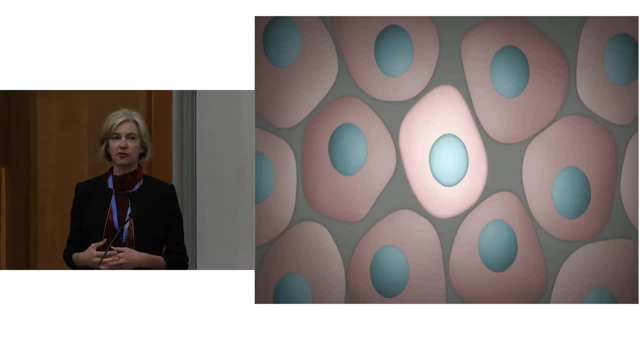 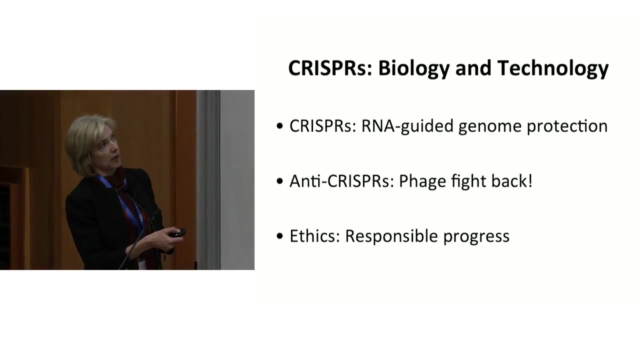 and has spread through many different areas of biology, enabling all sorts of research and now, applications that would have been very difficult, if not impossible, to do in the past. So I'm gonna just I really wanna tell you three things. I wanna talk a little bit about the mechanism of this process. 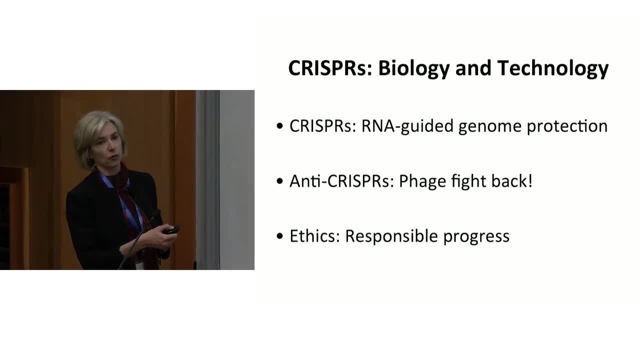 how this RNA-guided DNA cutting actually works. Why do we care? Well, you know I'm a biochemist so I think it's just kinda cool biology. But as you'll see, I think, once we understand how it works, 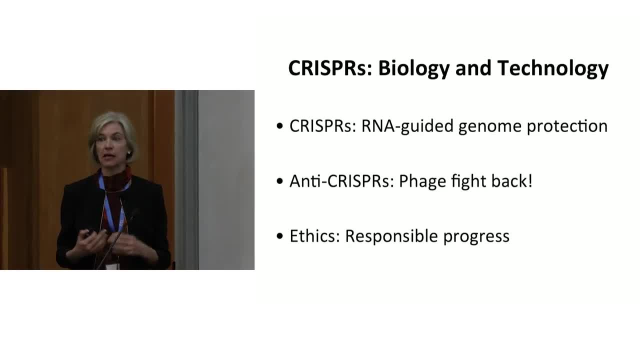 we can actually harness that activity and we can think about ways to make it better for applications that we wanna use it for. So I'm gonna tell you a little bit about this. I wanna tell you a little bit of new biology, So one of the things that's happening in the field right now. 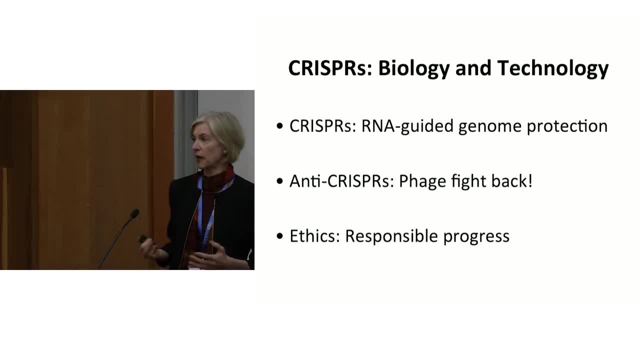 is continuing investigations not only of new CRISPR pathways, but also of how these are interfacing with other proteins that are found in bacteria, And one of the very recent discoveries has been the finding that many cells and the phage that infect them 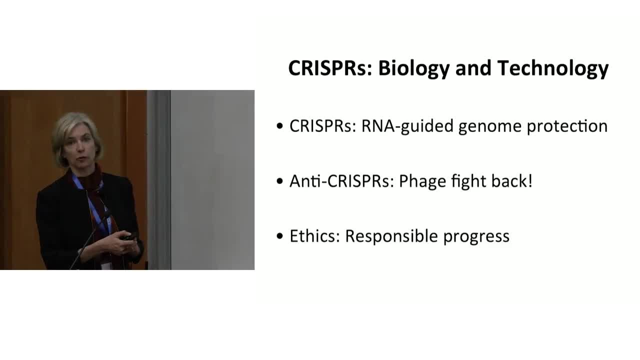 the viruses that infect them have what are called anti-CRISPR proteins. These are proteins that actually inhibit the CRISPR pathways, And these are turning out also to be potentially very useful as technologies, And I'll give you one brief example of that. 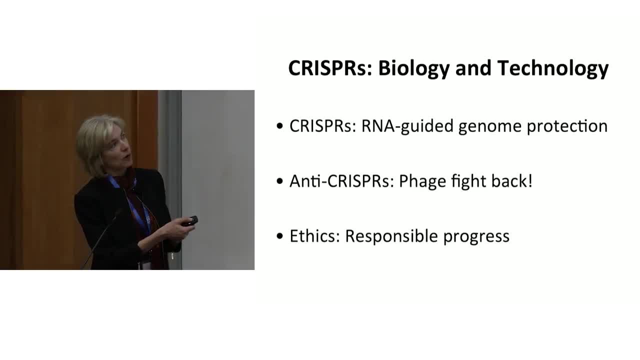 And then at the end I wanna just say a little bit about what we think about the societal implications of a technology that is so enabling for making targeted changes to the DNA of cells and organisms. It's really a profound thing if you think about it, right. 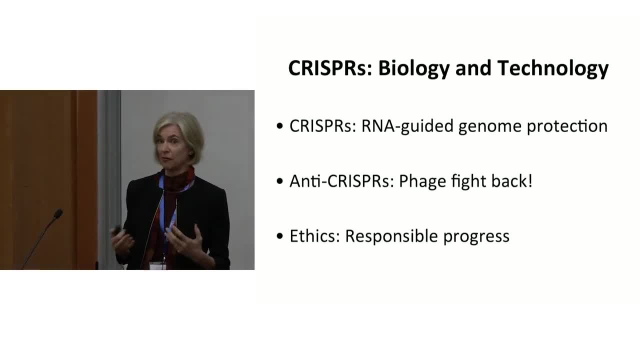 Because it really gives humans now the power to control evolution of organisms in our environment, and also potentially our own evolution, in a very targeted fashion. So it's exciting. it's enabling it's moving fields forward incredibly quickly, but it also brings sort of this sense of awe. 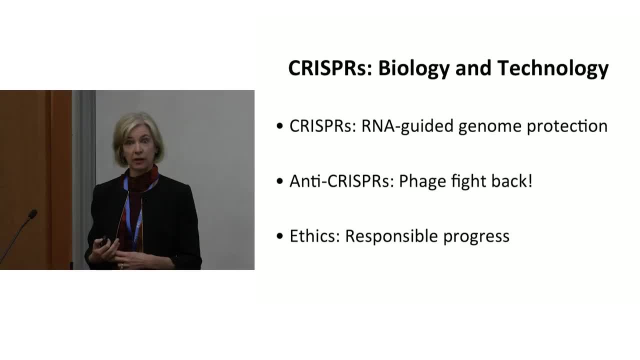 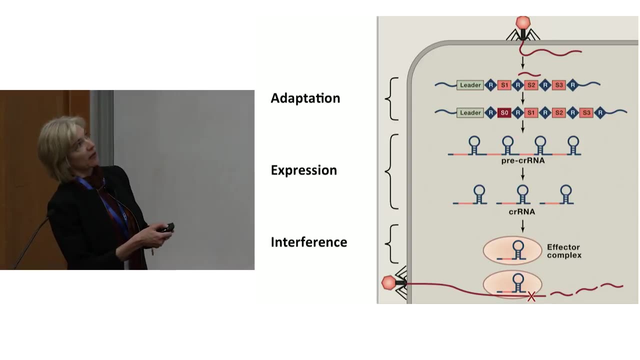 and the feeling that we need to proceed with appropriate caution and respect for this powerful technology. So I'm gonna say just a few words about that towards the end, Okay, but let's talk first about CRISPRs and how they operate. So this is a slide that shows the pathway. 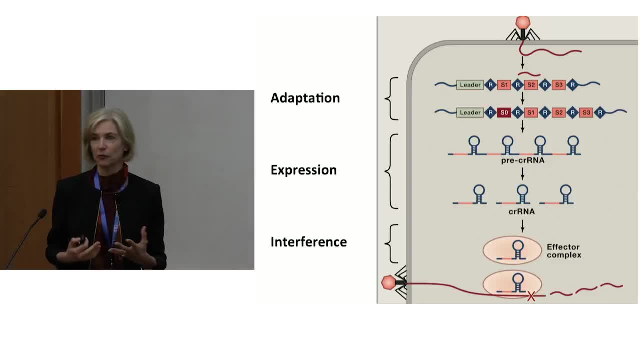 of adaptive immunity in cells. So one of the things that was very exciting in the very early days of the CRISPR field was the idea that bacteria actually have an adaptive immune system, kind of analogous to the way that we have antibodies. We have, of course, a very sophisticated 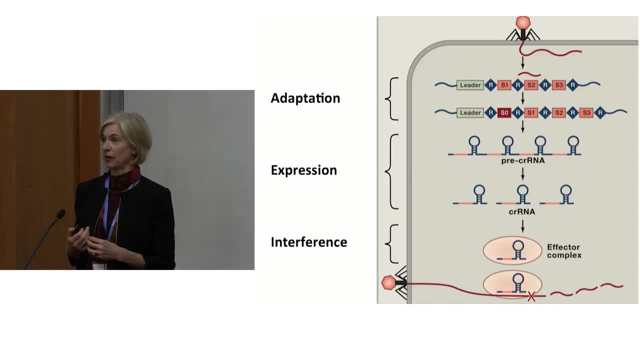 adaptive immune system that allows us to protect ourselves from pathogens. Nobody thought that bacteria, very simple single-celled organisms, would be capable of that kind of adaptation, but it turns out that they are. However, that pathway works very differently from the way that our own adaptive immune system works. 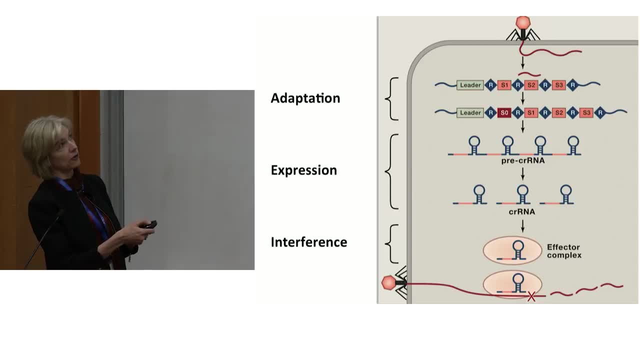 and it works by means of these acquired sequences that are integrated into the CRISPR arrays, as I showed you in that video, and then these become templates for RNA molecules that are transcribed that include copies of all of these integrated bits of viral DNA. 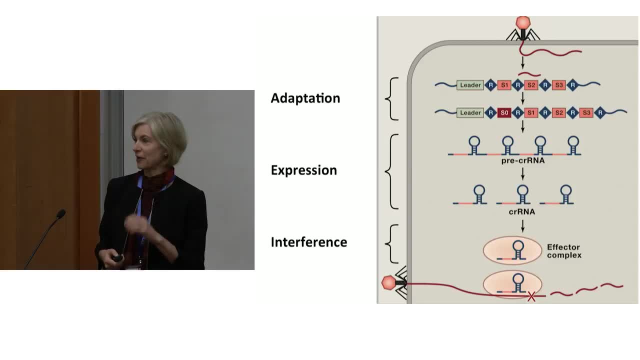 together with the associated repeat sequence, And note that, as the CRISPR acronym indicates, these repeats are often palindromic in character. That means that when they're made in a single-stranded form, like in the RNA molecule shown here, 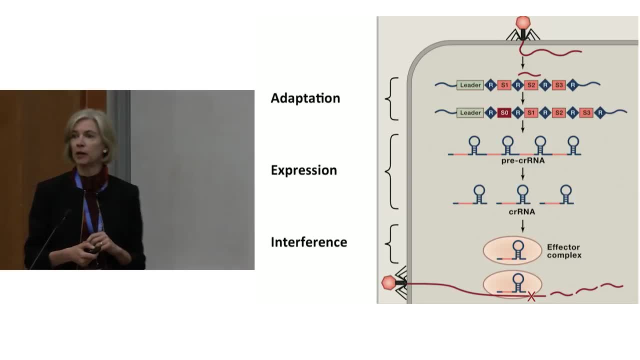 they can fold back and form structures like little hairpins that are recognized by some of the CRISPR-Cas proteins. and that's actually how these RNAs are often processed is by the recognition of those sequences. So the cell very nicely, kind of effectively labels these. as CRISPR RNAs. by using these unique sequence and structure tags, And after the RNA molecules are processed into individual units that each include a virally-derived RNA sequence, they combine with one or more Cas proteins to form surveillance complexes. They can search the cell looking for matching. 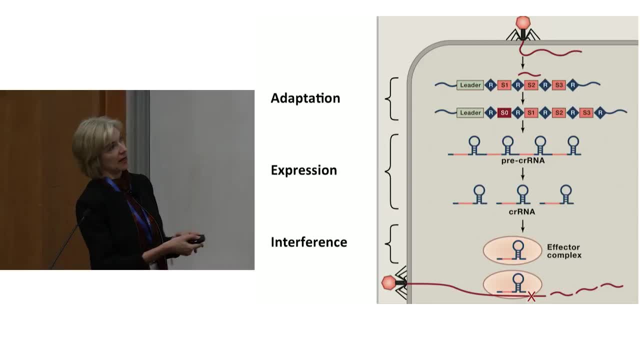 DNA or sometimes RNA sequences leading to degradation by cutting of those matching nucleic acids. So it's really a process of adaptation, acquiring these sequences from viruses that are entering the cell for the first time, expressing those sequences in the form of RNA. 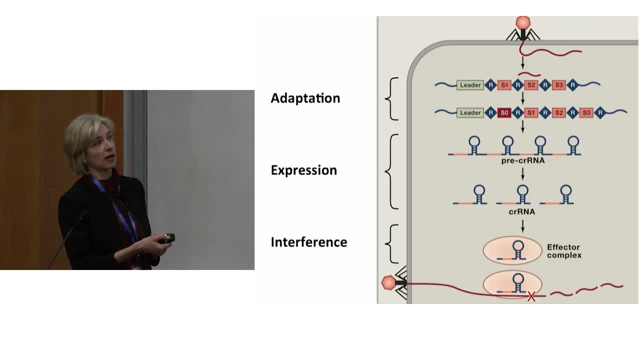 and then using the resulting protein RNA complexes to interfere with foreign nucleic acids. And so I'm gonna say, I'm gonna tell you a little bit more about this step here: interference, because this is really the step that, through understanding how it worked, 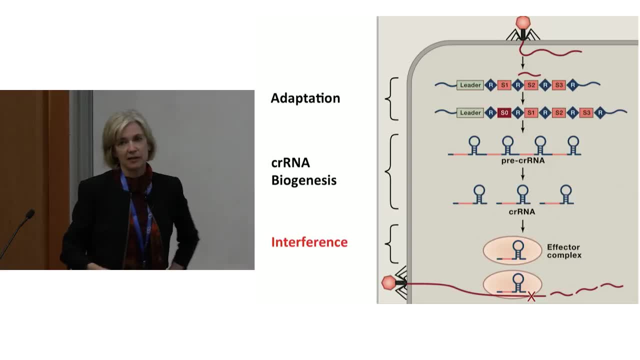 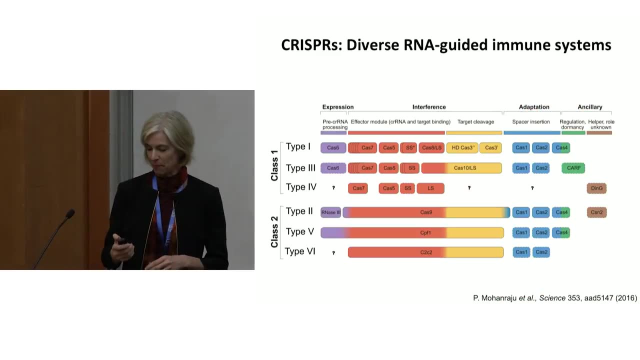 allowed this system to be harnessed as a gene-editing technology, as you heard about from Dana. Now, one of the things to appreciate about CRISPRs is that there are many flavors of these pathways, And this is a cartoon. it's actually already out of date. 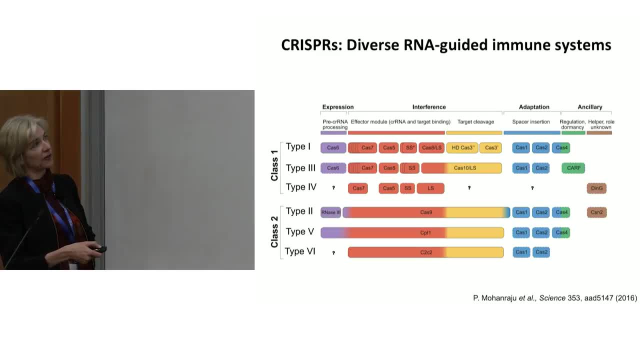 but it was taken from a review published in early 2016,. that shows different examples of CRISPR systems that are classified according to the numbers and types of Cas proteins that are found in these systems. And the main thing I want you to note here. 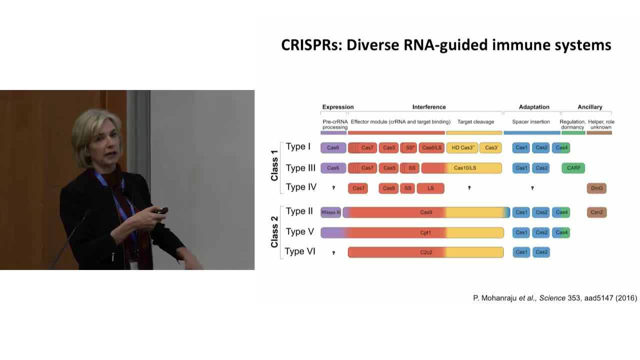 is that we can really classify these systems in two broad categories called Class I and Class II. The Class I systems all include multiple genes, multiple Cas proteins that have to be present in the cell and have to assemble with CRISPR RNAs. 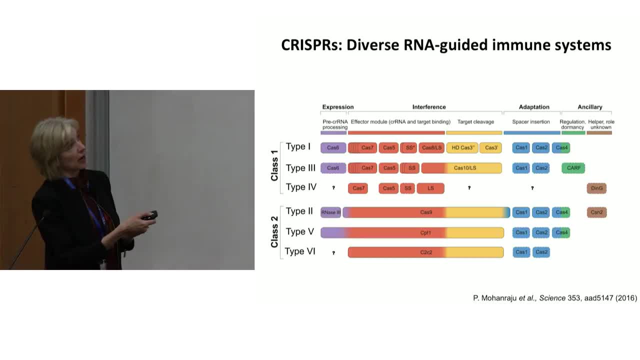 to form surveillance complexes. In contrast, the Class II systems of CRISPR systems include a single gene, typically that encodes one large protein that is able to combine with CRISPR RNAs and provide the cell with protection. And it was really through studying these systems. 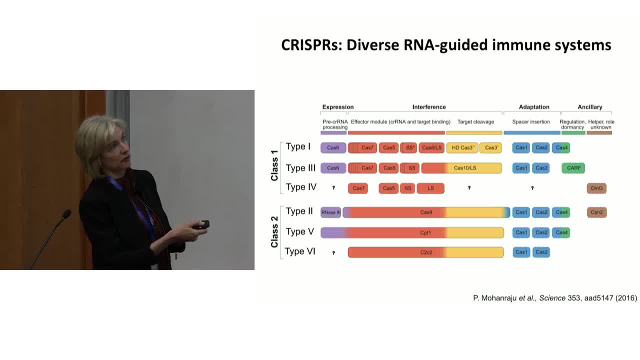 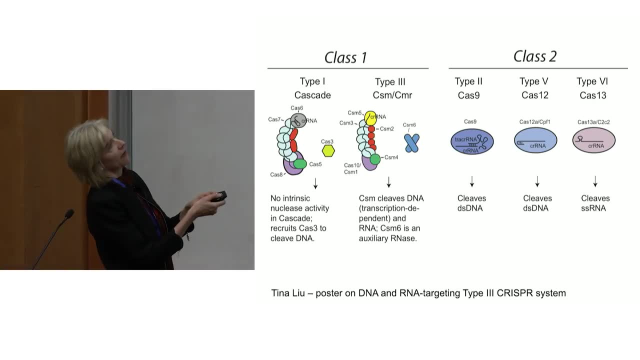 that it was possible to harness these genes, to harness these proteins for gene-editing purposes, And this is a slide that this is just showing. this was from a recent conference that we attended that really just shows examples in cartoon form of these different classes of systems. 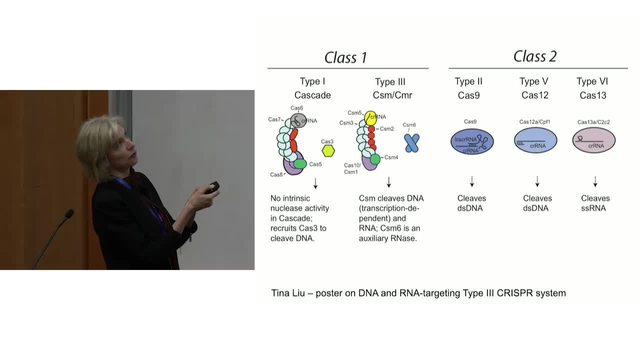 Class I over here, including large arrays of proteins that assemble with CRISPR molecules to form these surveillance complexes, And then over here, single proteins. They combine with RNA to carry out that kind of function. And so in the early days when research had focused, 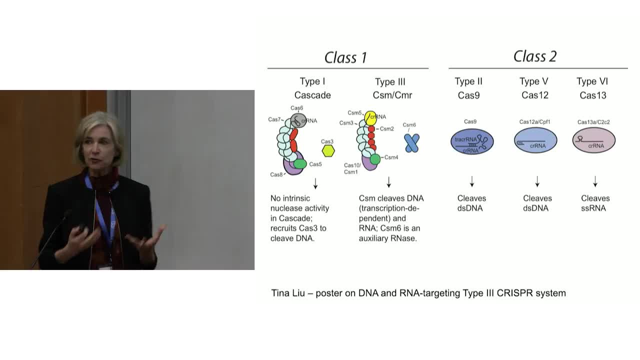 initially on these Class I systems. they were very interesting, the functions were fascinating, but it was hard to imagine how you could really harness them as a technology, because you would require multiple proteins to be made in cells and to assemble and it just seemed like a many-component system. 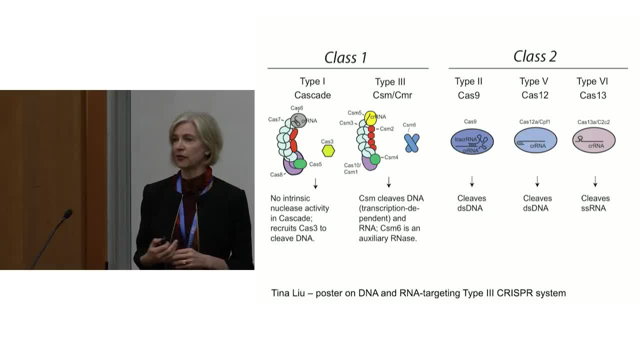 that might be very complicated to get working in a heterologous cell type, Whereas with CRISPR you could have multiple proteins. you could have multiple proteins. you could have multiple proteins. work on these systems over here which are much simpler. 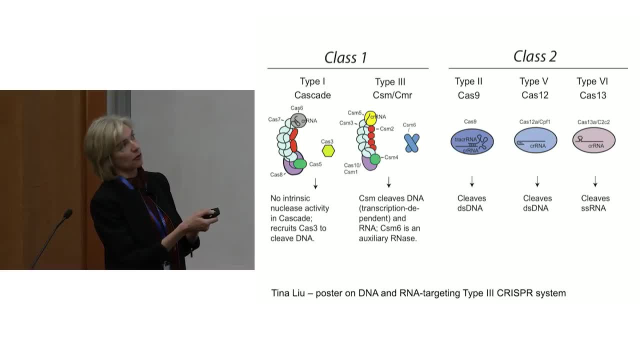 and were simplified further by understanding that you could combine the two natural RNAs called CRISPR RNA and tracer RNA into a single guide form. This converted what had been initially a very looked like a pretty complicated kind of system into something that looked a lot easier to harness as a tool. 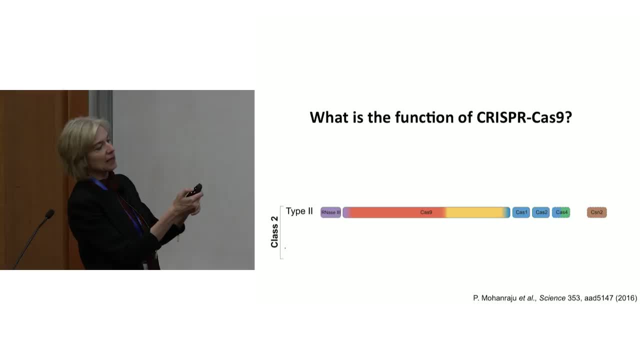 And so, for us, one of the key questions that we set out to address in those kind of early days was to understand the function of the first example of this large type of protein- single protein- in the Class II CRISPR systems that could operate. 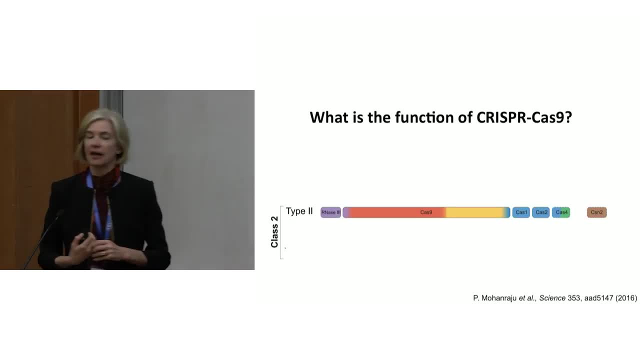 to protect cells in an RNA-guided fashion, protect them from viral infection. And the question was really: what is the function of this encoded protein which in the very early days was known as CSN1, and then very quickly became called Cas9.. 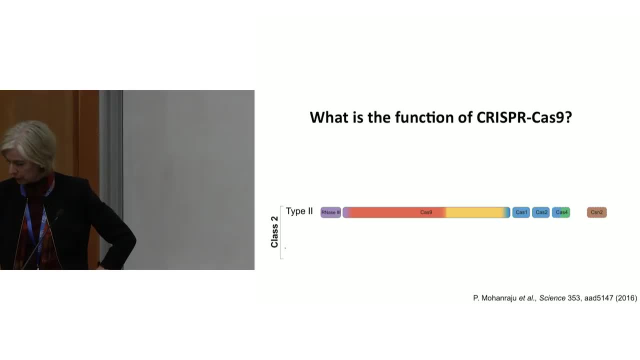 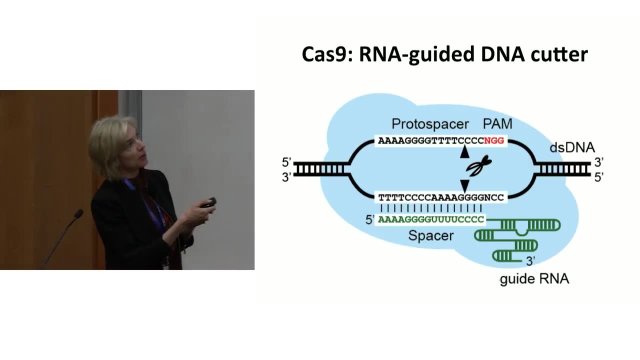 And that line of research, which was conducted with a collaborator, Emmanuelle Charpentier, and her student, Krzysztof Czajlinski, revealed that Cas9 is an amazing enzyme that has the ability to recognize double-stranded DNA. 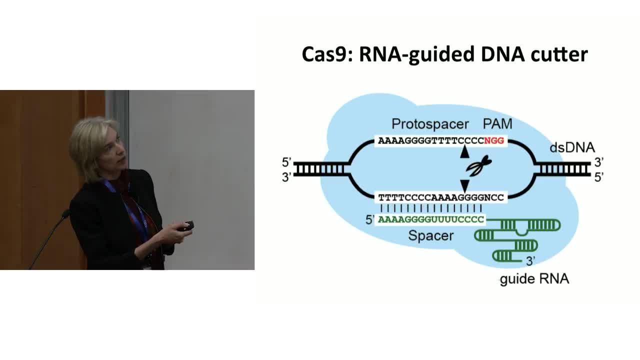 at positions in the DNA sequence that match a 20-nucleotide sequence in this guiding RNA. And note that I'm showing you here this, the guide RNA in its single guide form, where the natural CRISPR RNA, which would be this part of the sequence here. 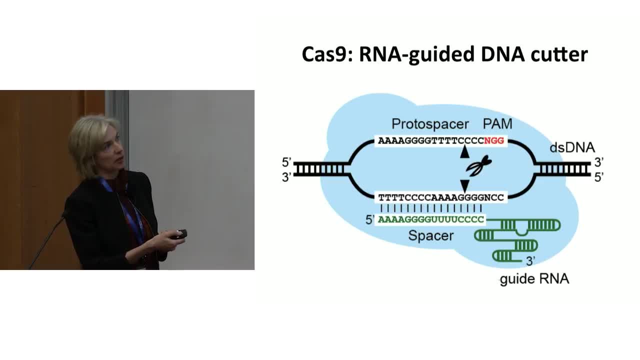 and what's called the tracer RNA, which would be this part of the sequence over here, have been combined by linking them together covalently, So this can be made as a single transcript, something that turned out to be very helpful in harnessing this as a technology. 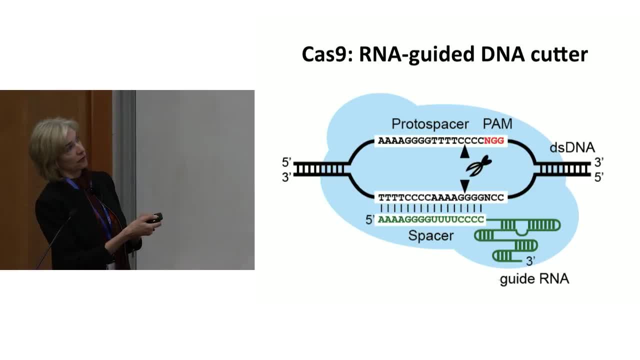 because it's made it easy for researchers to make RNAs that would have a desired sequence here. that would track Cas9 to a particular sequence or a site in a genome and trigger its DNA-cutting ability, allowing it to make a blunt double-stranded break. 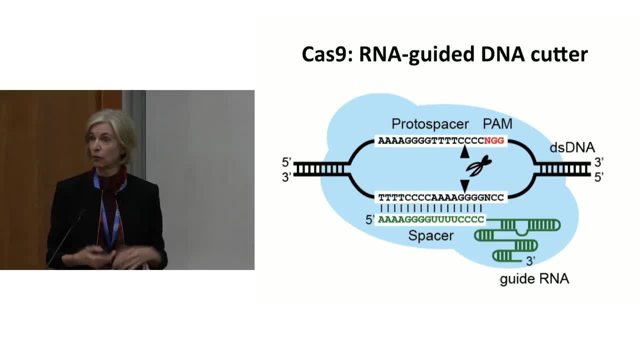 at a precise place in a DNA molecule or in an entire genome, And you've already heard quite a lot about that from Dana. And so in our lab we've been sort of curious about really addressing this question of how recognition really works. 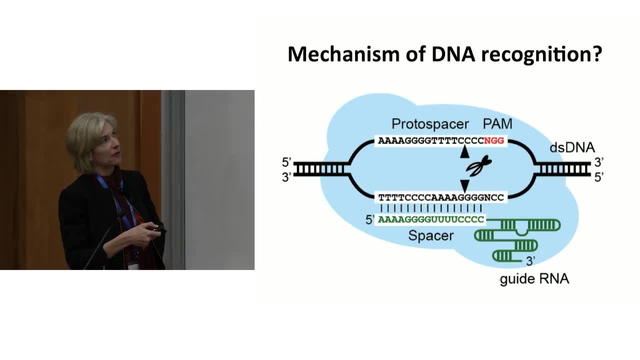 not just that we can see that. okay, it involves base pairing, but it's really also a question of how this protein is able to open up the DNA in a genome, And you've got to imagine that you've got the DNA in a typical eukaryotic cell. Of course it's in the nucleus. It's also highly packaged. It's wrapped around histones. It's compacted into chromatin- different types of chromatin. Lots of proteins around are bound to it. DNA replication and repair machinery and other proteins moving through. 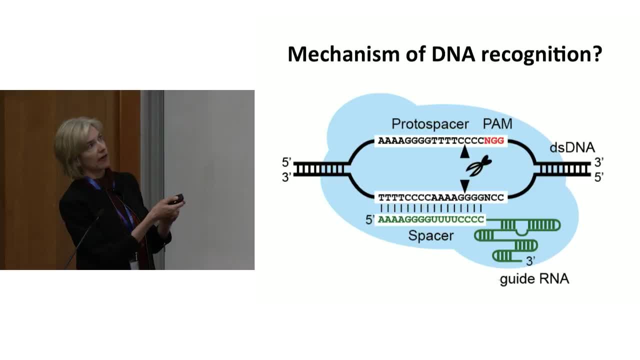 How does this bacterial protein deal with all of this And somehow find these sequences typically quite accurately and generate double-stranded breaks? And that's really the question that we've been seeking to understand over the last few years, And I threw this slide in to remind me, to tell you. 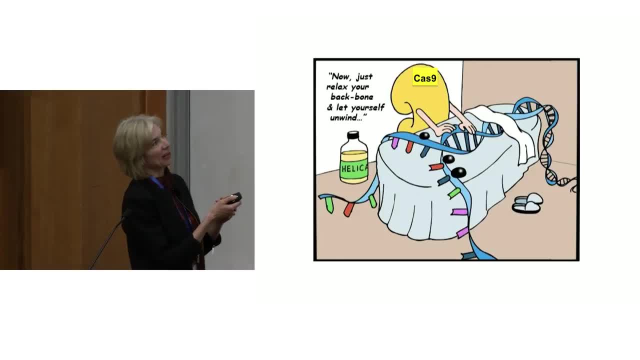 that, unlike this sort of cartoon right here, the Cas9 protein has to be able to unwind DNA without any kind of replication, So it can unwind DNA without any external source of energy, So it doesn't hydrolyze ATP or GTP to unwind DNA. 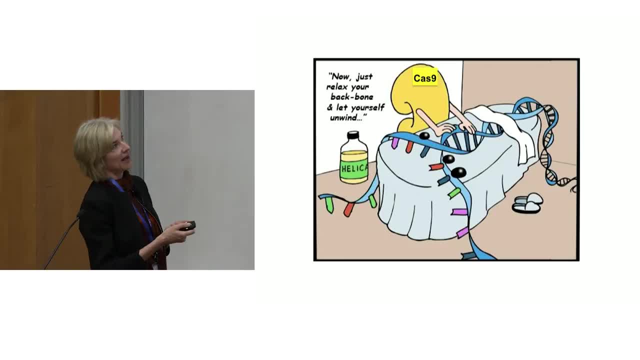 Somehow it triggers DNA unwinding by some other mechanism, And so we'd like to understand how that works, And why do we want to know this? Well, again, we're very interested to understand what makes this enzyme functional in eukaryotic cells. 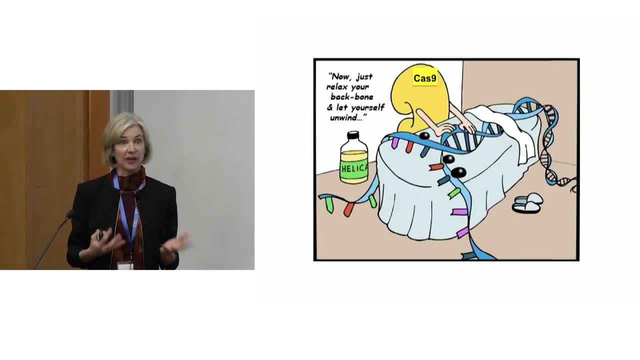 How does it deal with chromatin, et cetera? How does it get to the right site in the cell? What happens when it gets to the wrong site? Can we do things to prevent it from accessing the wrong site? make it even more accurate than it is, naturally? 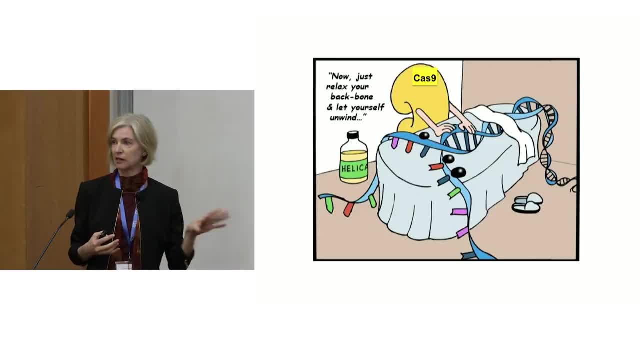 And also can we harness its DNA recognition activities to do other things, like not just trigger covalent changes to the DNA in a genome, but also to recruit other factors to positions in a genome. Use it for DNA imaging, for example. 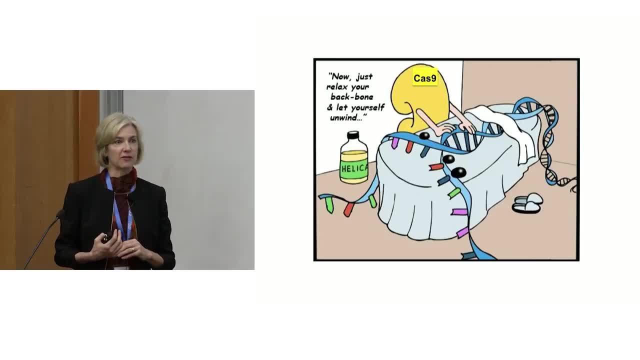 and also for the kind of thing that Luke Gilbert is doing, which is harnessing its activity to regulate the expression of genes, So making changes to the levels of proteins in cells without actually changing the DNA sequence in cells. So one of the things that's emerged over the last few years. 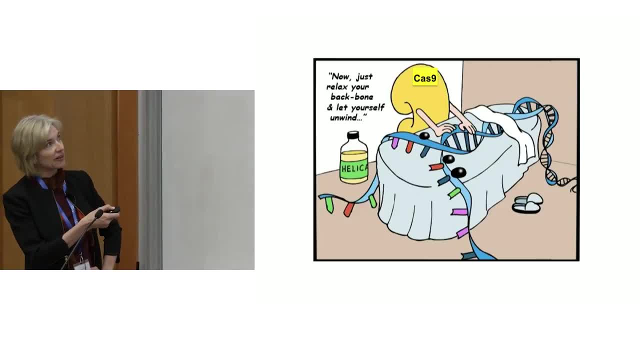 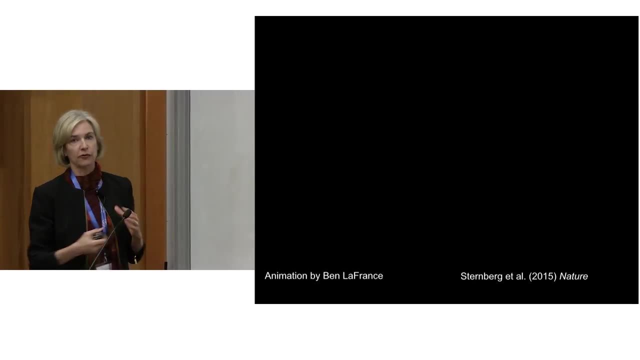 is that one of the ways that Cas9 probably does this is through its ability to change conformation upon binding to nucleic acid, And so I'm going to show you a little video that was made by a student, Ben LaFrance, that morphs together a series of crystallographic structures. 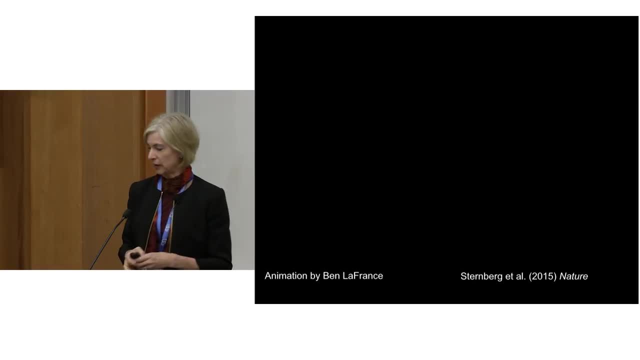 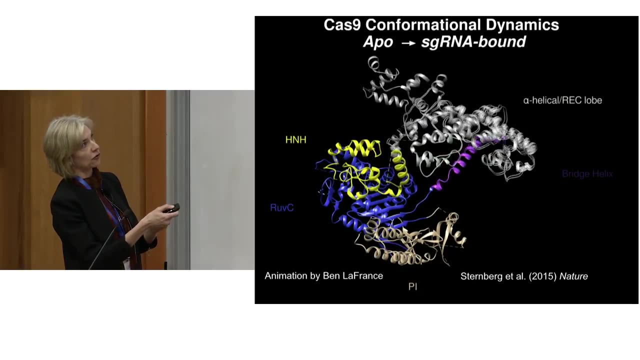 solved for Cas9 in different states of assembly with nucleic acid, And so this is a movie that starts with Cas9 protein alone. that's a crystallographic structure and you see it morphing to the state of the protein when it's bound to the orange guide RNA. 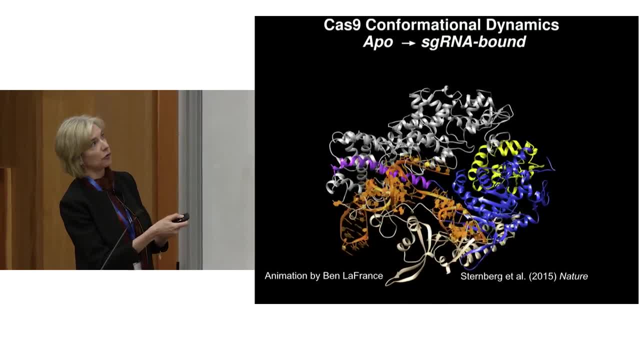 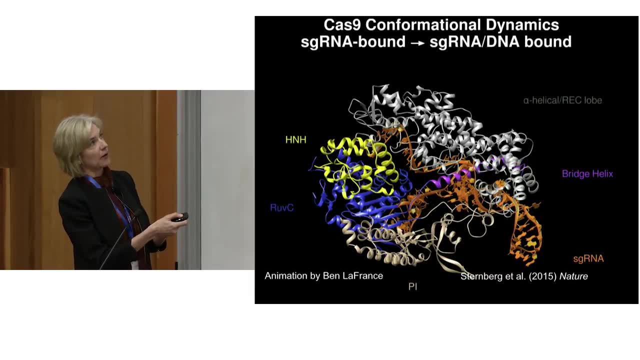 And you saw a big rotation in this gray part of the protein. that reorients it to open up a channel in the center where the guide part of the RNA is sitting, And then, when this protein binds to a DNA molecule, you can see additional structural changes. 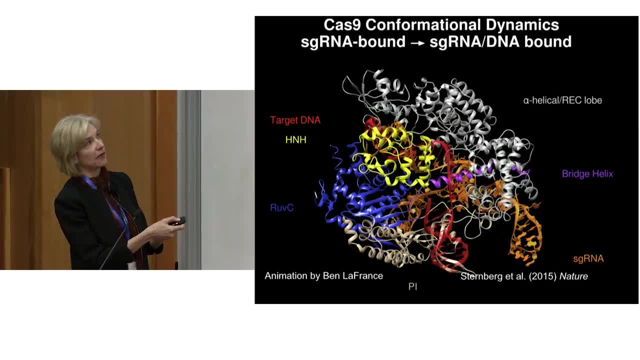 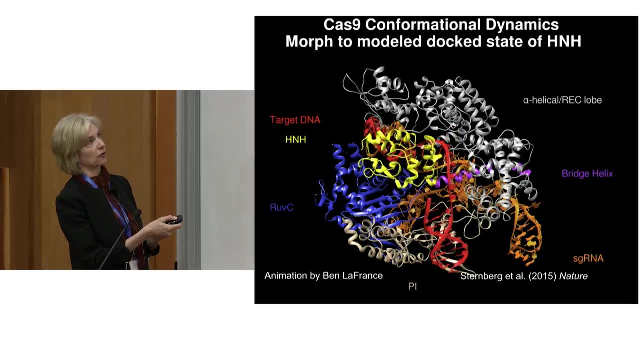 that happen in the protein here to accommodate the RNA-DNA hybrid that forms Now those structures showed us that there had to be an additional structural change, This rotation that you're seeing right here, which was modeled in at the time that we made this video. 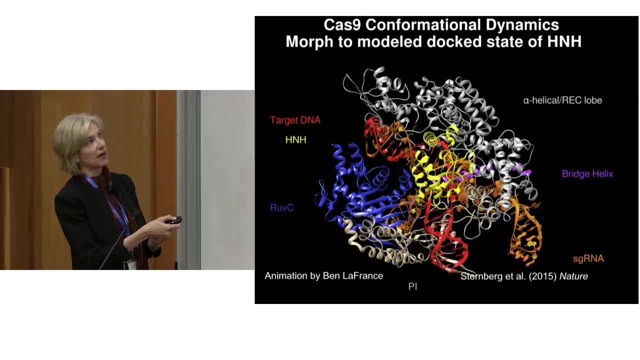 because we knew that this part of the enzyme, which is a domain in the protein called HNH- this is actually one of the chemical cleavers in Cas9. It's the part of the protein that cuts the DNA strand. that base pairs with the guide RNA. 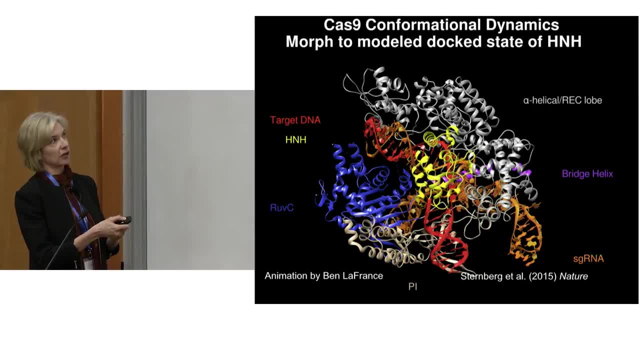 But in all of the crystal structures that were solved initially, which were solved using single strands of DNA that were annealed to the guide RNA, this domain was not in the right place to actually cut the DNA. It was located quite far away. it was sort of over here. 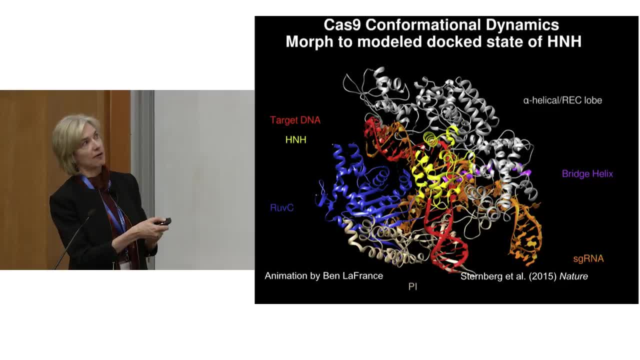 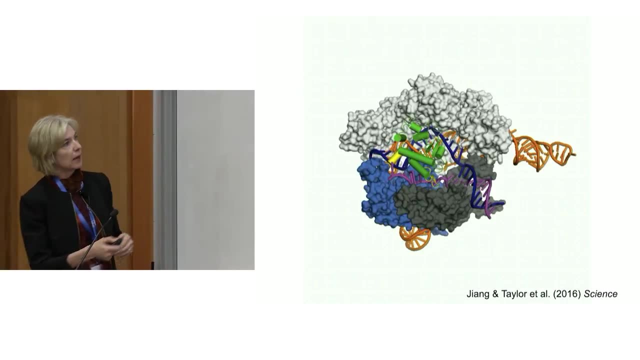 rather than in this position. you can see modeled here where it would have to be positioned to actually make a cut in the targeted DNA strand. So what was going on? And so one of the things that emerged more recently in research that was done by a team at Berkeley- 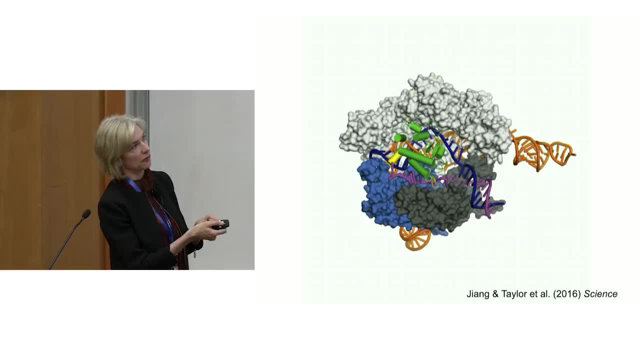 including Fugo Zhang and David Taylor in my lab, and this was a very nice collaboration with the lab of Evo Nogales here at Berkeley, who does cryo-electron microscopy. was that a combination of crystallography and electron microscopy allowed these students? 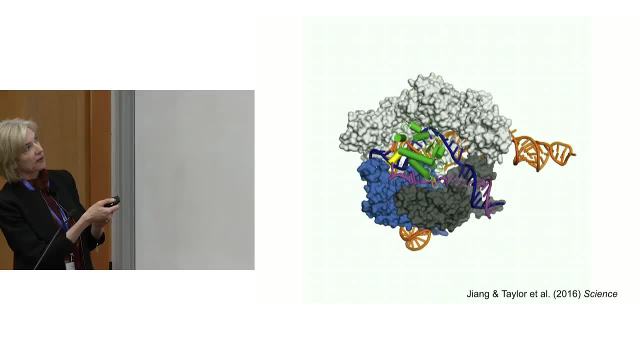 to trap a structure of the Cas9 protein bound to its true substrate, which is a double-stranded DNA molecule, And so you can see that hopefully it's a little bit dark here, but hopefully you can see this double-stranded DNA. 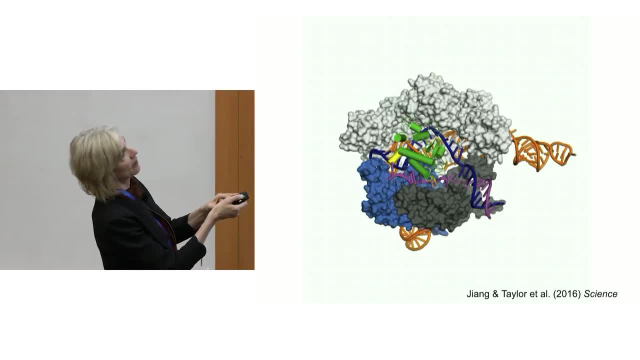 So here's: the one strand is in blue and the other strand is in magenta, So you can see the duplex DNA here opening up inside the protein. This targeted strand is forming a duplex with the guide RNA. And then here's the non. 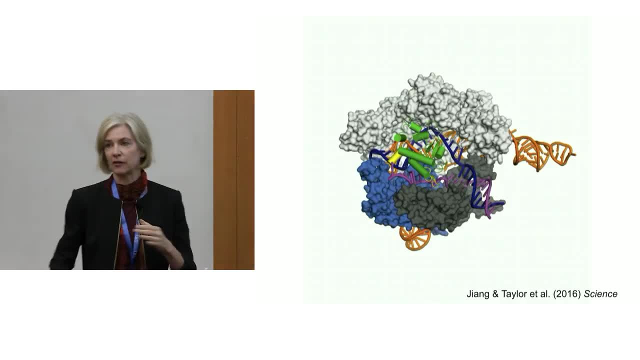 what we call the non-target strand is over here, And you remember that when Dana Carroll talked about work that Chris Richardson is doing at the IGI with Jacob Korn, they had found experimentally that this part of the DNA is more exposed after DNA cleavage. 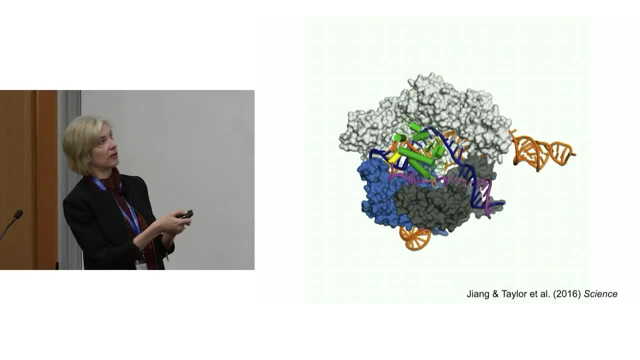 And this structure kind of reveals the basis for that. You can see, it's located really on the surface of the protein rather than buried inside like this strand over here. And the cool thing about this structure was that we found that the- and I think I this is actually an animation. 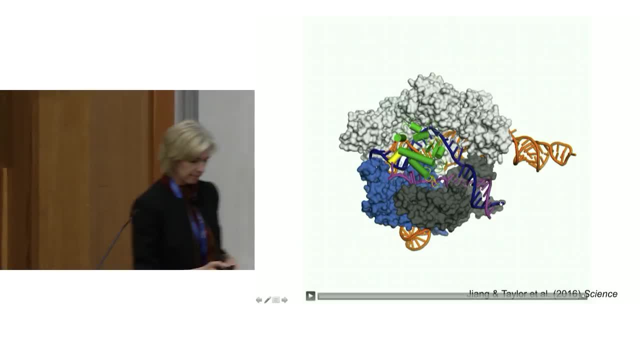 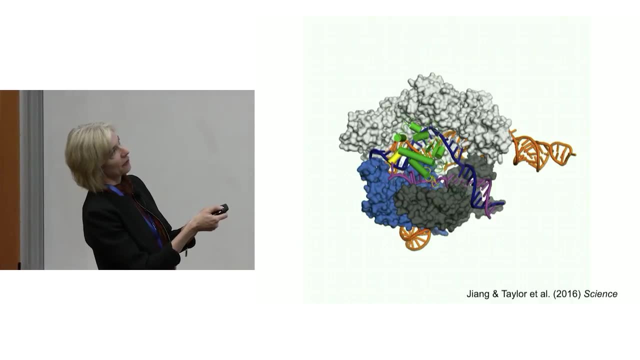 I could show this to you, But it's basically, I think I'll just tell you that this is a. if you look at this green part of the enzyme here in this structure, this domain that cuts the target DNA strand is now actually positioned very near. 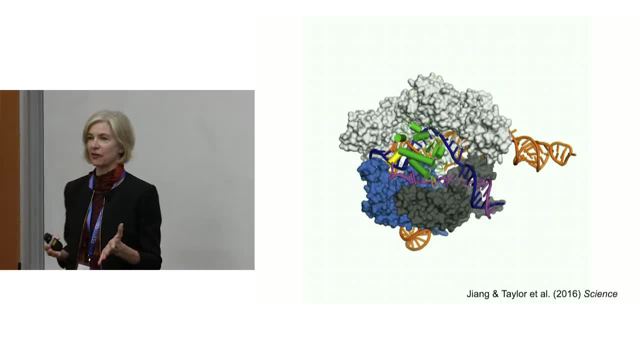 where it needs to be to cut the DNA. So there's something about having the non-target strand present in the complex that actually triggers this protein to be in the right conformation to actually conduct chemistry. And so we're- you know we're- doing a lot of work now. 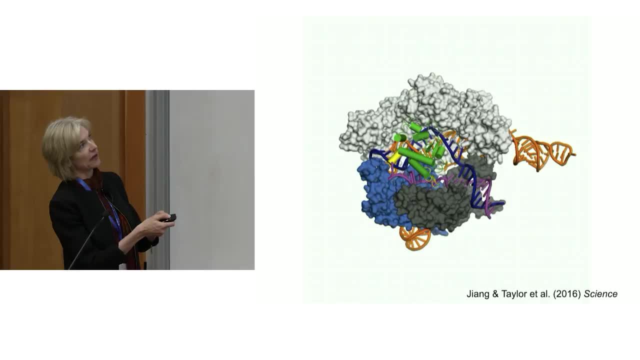 and I'll tell you a little bit about this shortly- to really understand what triggers this domain to swing into place, to cut the DNA, because there's a lot of evidence that this is a protein that can bind DNA quite readily, even in cells. 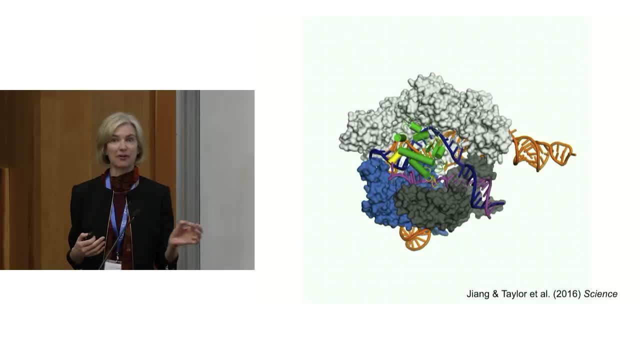 and people have done experiments showing that you can detect binding of Cas9 at a lot of sort of close but not quite perfect matches to the guide RNA in cells, and yet most of those sites are never altered chemically. Why is that? Well, we think one reason is because 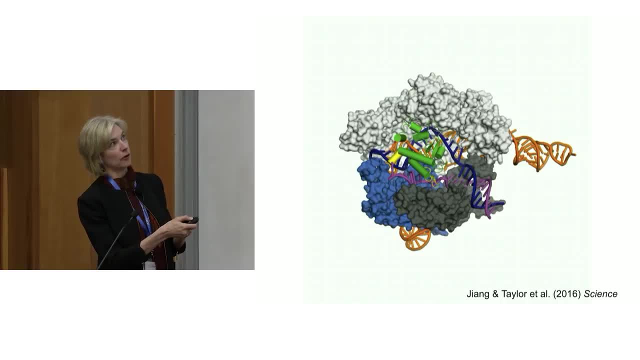 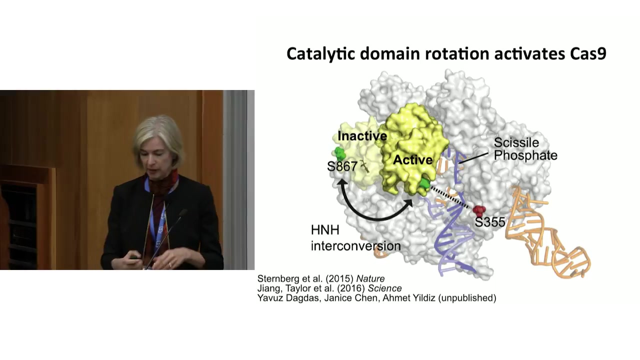 this domain is actually very sensitive to full base pairing of the guide RNA with the target DNA sequence. And just to show you how we, why we think that's true, I'm gonna show you one series of experiments that are being done to test the conformational states of Cas9. 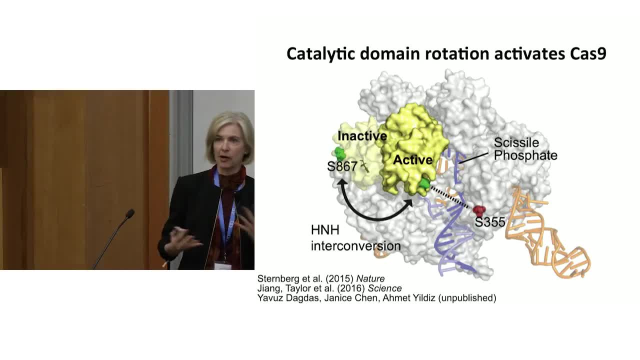 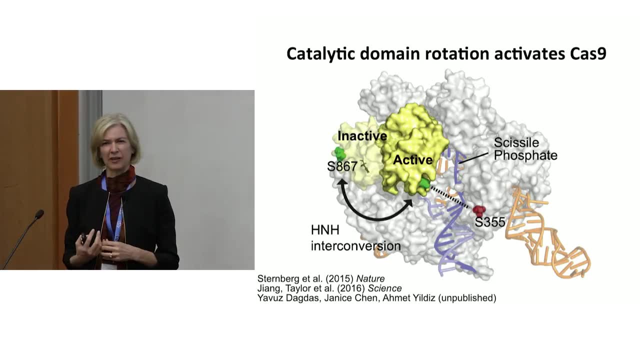 So you might, if you don't do biochemistry or think about proteins in this way, you might wonder: how do we know that? How can you actually figure out structural changes in proteins? I mean, that sounds kind of kind of detailed and certainly we can't get that. 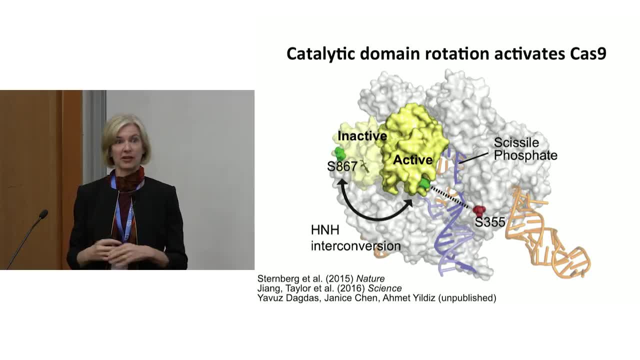 information necessarily from snapshot structures, like we see in crystallographic structures of proteins. And so one strategy for testing conformational changes in proteins takes advantage of the real physical changes in distances between atoms or individual amino acids in a protein. if there's a change, 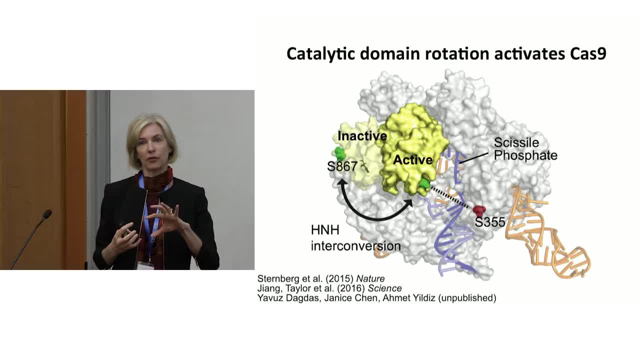 in its structure. And so when we had this model for what we thought must be happening in the Cas9 protein with respect to this active site, this HNH domain that had to swing into place to cut the target DNA strand, the idea here was to 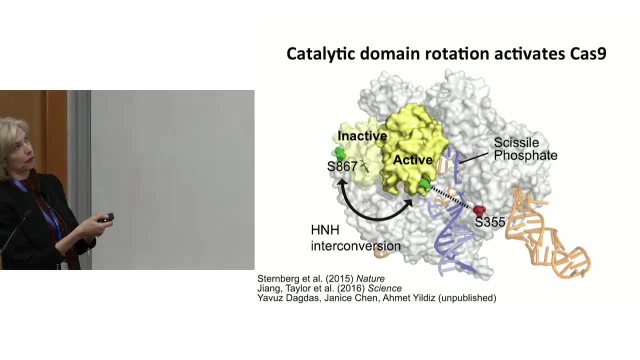 introduce pairs of chemical dyes on the surface of the enzyme that would be in very different spatial relationships depending on the conformational state of Cas9.. So this is just showing an example where we have this HNH domain in yellow. so the inactive state. 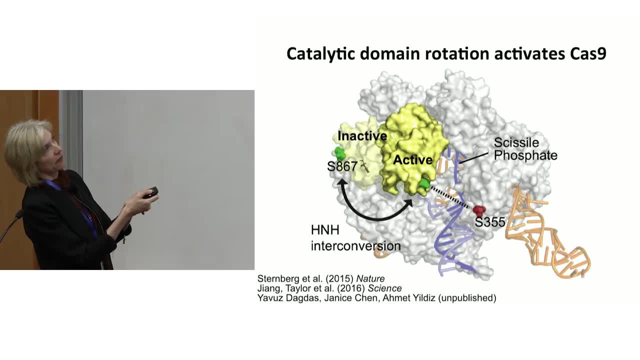 is shown over here, We've got a dye sitting right there. When this domain swings into the active position shown here, you can see that the position of that dye moves quite a lot. And if you've got another dye sitting over here in the protein, 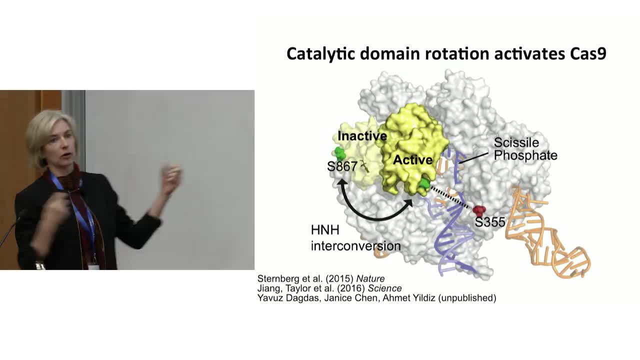 these two start off initially very far apart. They can't really chemically interact, so you don't get much of a signal by something called resonance energy transfer. But when this domain change happens. now these two dyes are very close together and you can detect. 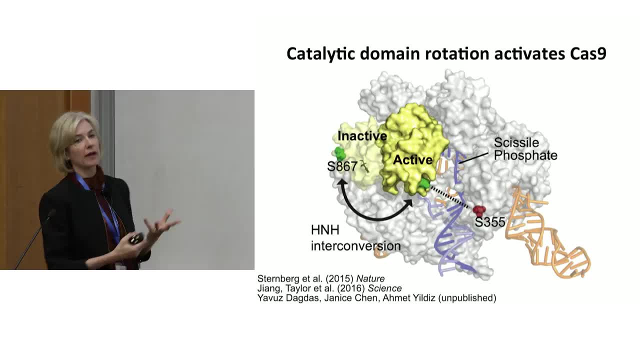 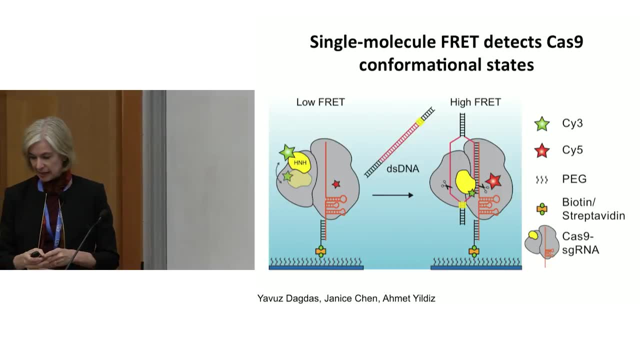 a resonance energy transfer between the two. So that's one way that you can detect these kinds of structural changes. Just to show you a little bit of data. this is actually fairly new. I don't think this publication has appeared yet, And this is a collaboration with. 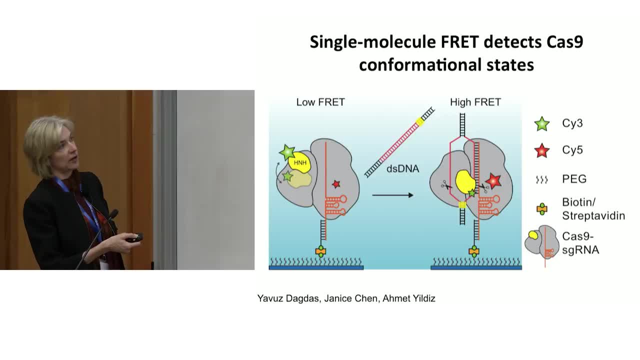 Ahmet Yildiz, a biophysicist here at Berkeley, and his student Yavuz, and a student, Janice Chen, in my lab. What these students did was they were able to set up a system where they can tether the Cas9 guide RNA. 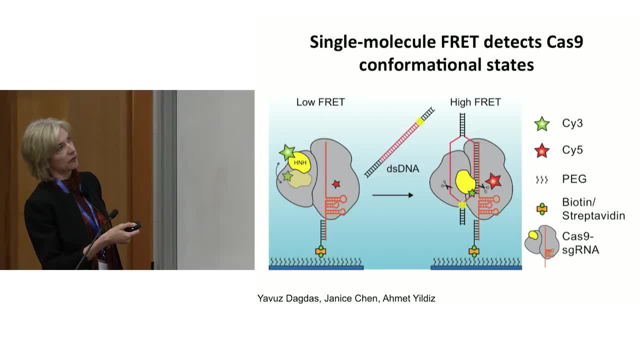 complex to a surface And they do this by. so here's the guide RNA. You can see its RNA end is being chemically linked to this slide surface And then we can flow in double-stranded DNA substrates for a recognition by this complex And 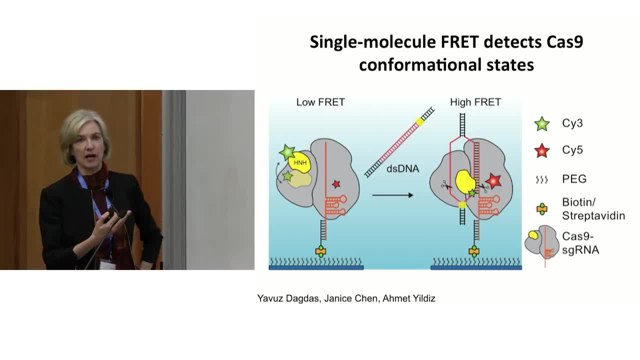 we are using Cas9 proteins containing these pairs of dyes that I showed you, So we can actually monitor changes in fluorescence resonance energy transfer, called FRET, as a function of interactions with these DNA substrates And by setting up an experiment like this. it's very trivial. 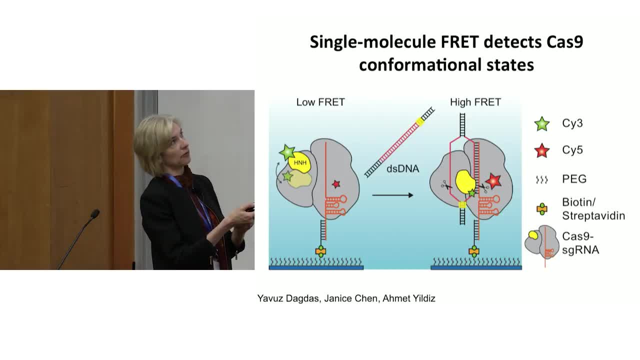 to change the DNA sequence So we can have DNA molecules that have a perfect match to the guide RNA. and then we can also test DNA molecules that have various mismatches to the guide RNA and see how that affects the ability of the protein to interact. And I'll just 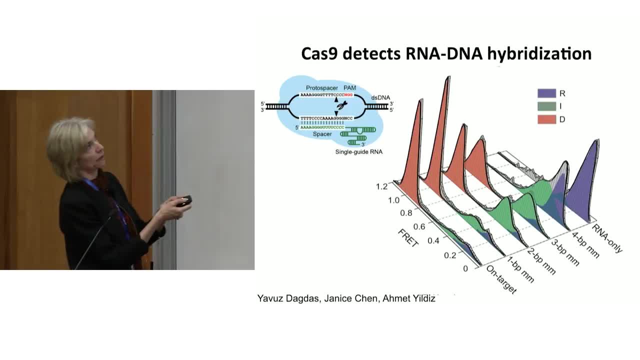 show you a little bit of data. So what does the data for these experiments look like? So here we've got the Cas9 RNA DNA complex that we're monitoring formation of, And over here you can see, we're plotting the resonance energy transfer signal. 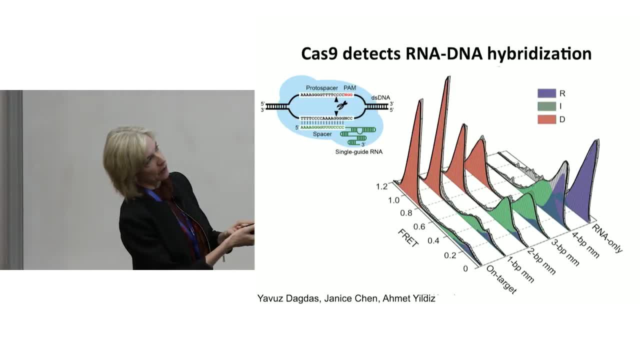 that we're getting as a function of the complementarity between the DNA molecule we're using in the experiment and the guide RNA. So if you just look at this last line here, this is what we see if we use just the Cas9 RNA complex. No. 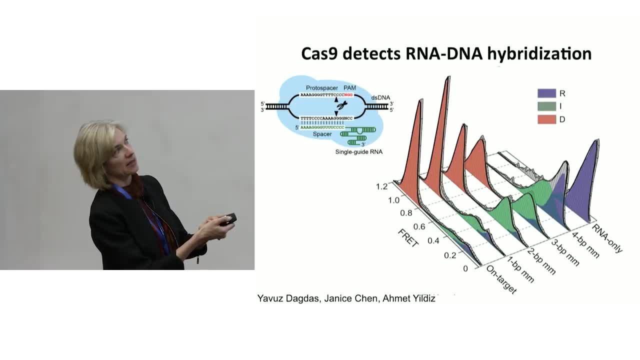 DNA is present. The protein is in an inactive state, as I showed you before, And we get a FRET signal that so most of the particles here have a very low FRET signal. That's because the dyes are very far apart in that conformation. They don't 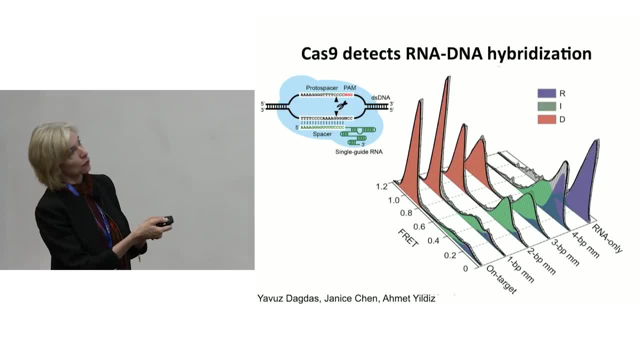 interact. As we add DNA molecules that have increasing amounts of complementarity, all the way up to a perfect match to the guide RNA, you can see that more and more of the molecules are populating this active state where the dyes now are very close together. because this: 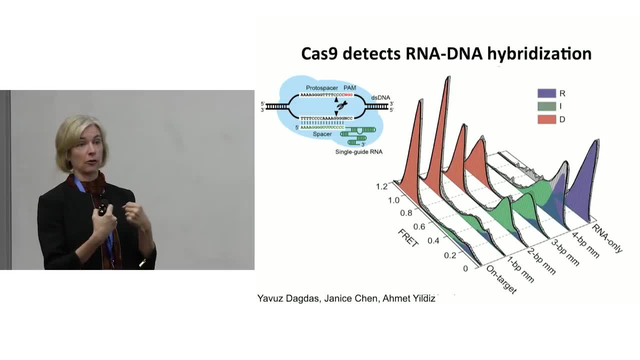 conformational change has happened And so we're getting a very strong signal between the dyes. So we can really monitor that very nicely. And the cool thing in this experiment was that we found that a lot of the molecules- initially these proteins- get stuck in an 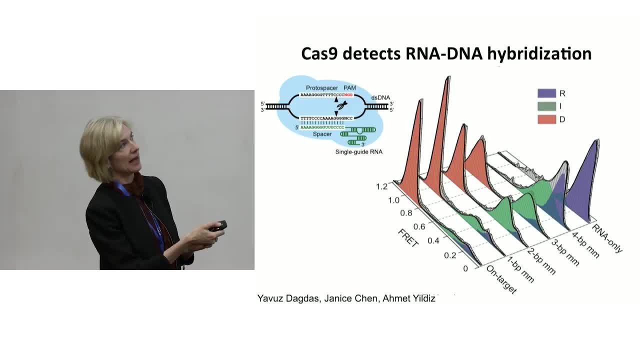 intermediate conformation. It's not fully off, it's not fully inactive, but it's also not in the active state either. So there's sort of this intermediary state that is populated and sort of the degree of population of this state depends again on the complementarity. 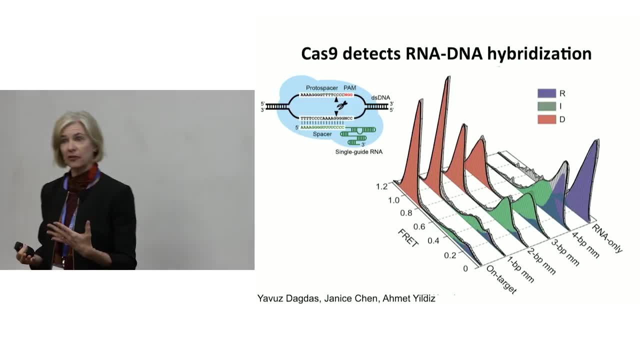 between the DNA and the guide RNA. So it really tells us that this is a protein. that's a sensor, right. It's really sensing the degree of a match between a target DNA and the guide RNA And that sensing is being conveyed in terms of this conformational change. 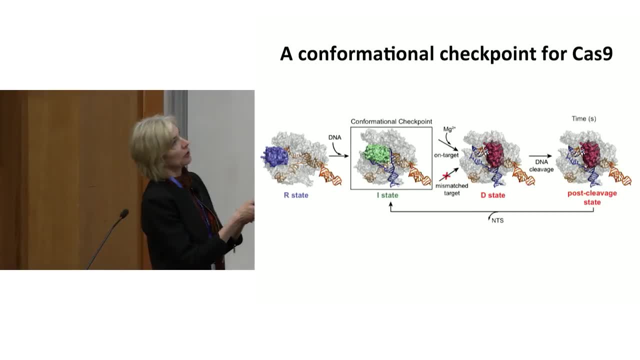 of the protein, And so that really led to the idea that the protein goes through this series of steps to get to an active state in which it starts off in this inactive form. it goes through an intermediate and then it reaches this sort of fully docked state. 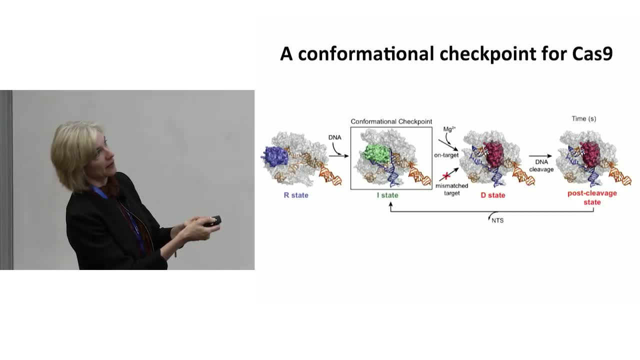 and then is able to cut the DNA and this can then dissociate and sort of the protein gets reset and can cut other DNA molecules in sort of a catalytic fashion. And what we're doing right now is we're actually using this to design versions. 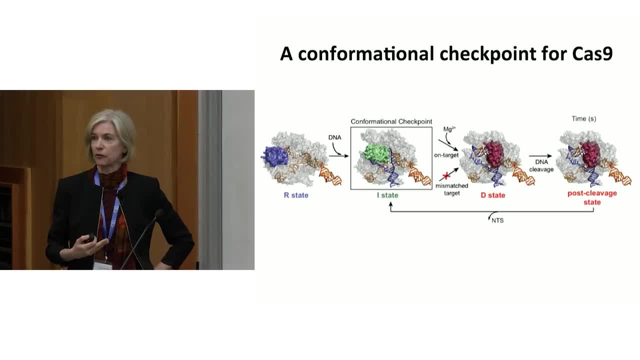 of this protein that are even more accurate. they're even better sensors of the target DNA than occurs in nature, And we have a paper that we just posted on the bio archive, a preprint server, that shows design of new mutations in the Cas9 enzyme that we think. 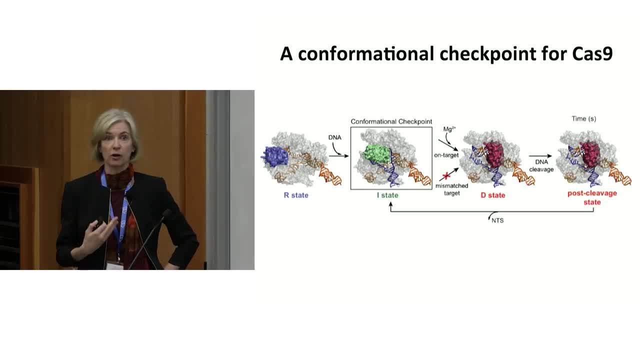 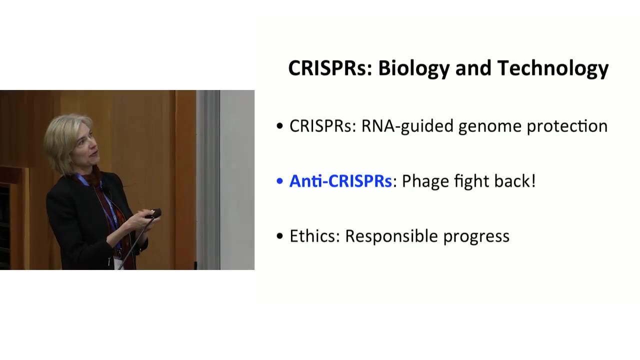 are making this protein an even better sensor, potentially more accurate at DNA cutting and thereby maybe useful as a technology for gene editing as well. Okay, so let's talk a little bit about how nature fights back. And so the story of anti-CRISPRs really started. 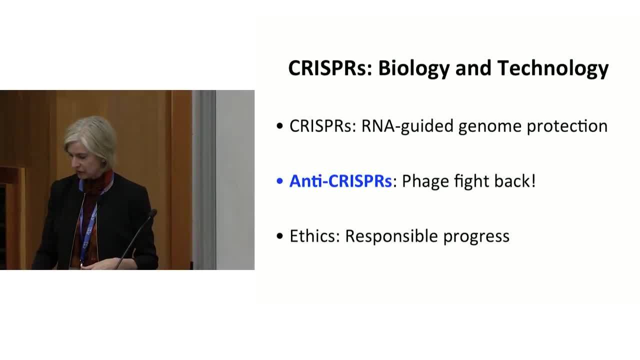 kind of where the story of CRISPRs did, which was with microbiologists who were trying to understand how these systems operate in nature and, of course, when there's a sort of ongoing battle between infectious agents and their host, they're going to be. 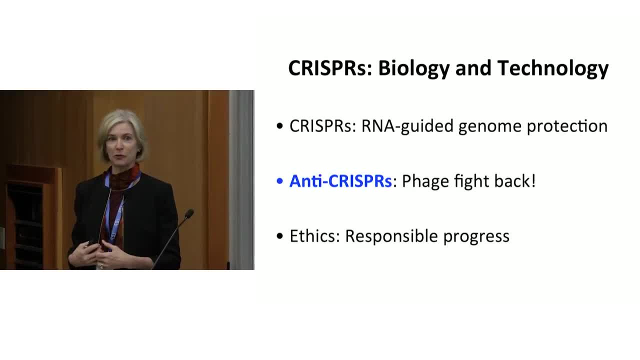 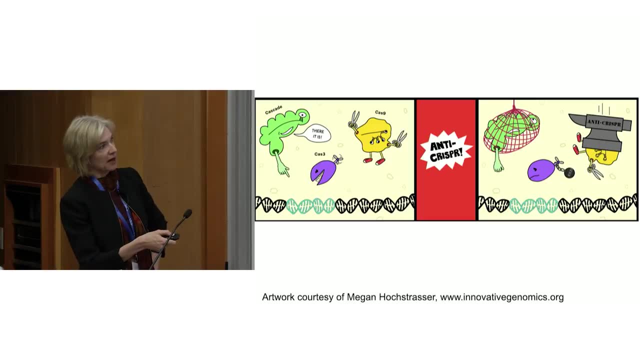 protein. there's a lot of selective pressure for both systems to evolve ways to get around the defenses that are put up in each case. This is a cartoon that was actually made by Megan Hochstraser, who is one of our outreach coordinators here. 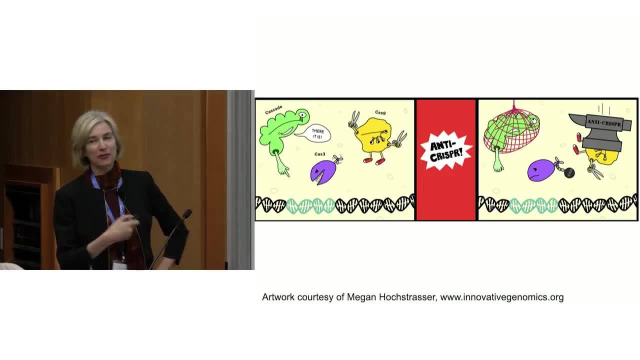 at the IGI illustrating sort of, in fanciful form, different ways that we could imagine that cells might come up with ways of blocking these CRISPR pathways. They could have ways of stopping the CRISPR proteins. they could prevent binding to the RNAs. potentially, 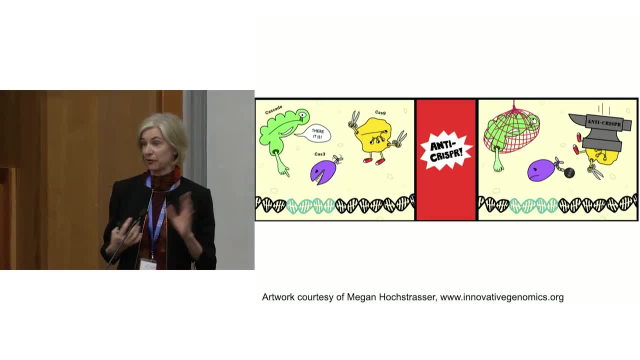 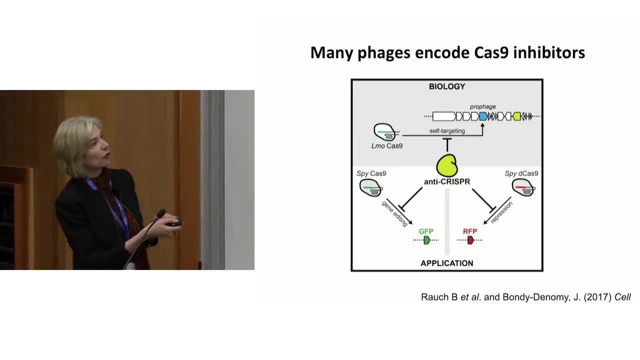 and there might even be other pathways, as I'll show you, that would lead to inhibition of CRISPR systems, And so Joe Bondi-Dedemy, a scientist at UC San Francisco across the Bay, is one of the lead scientists who's been working on these. 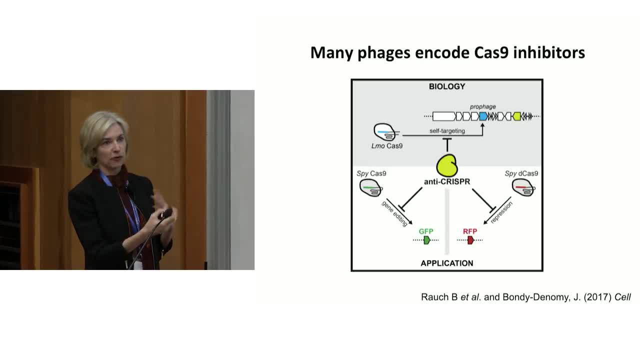 multi-CRISPR systems. So he's a microbiologist studying ways in which phage interact with their host bacteria and he noticed that there were sort of interesting examples of organisms that should have been, or phage that should have been eliminated by these CRISPR pathways. 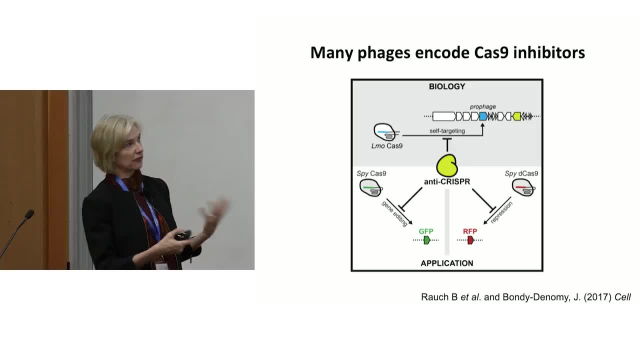 that weren't somehow. And so why was that? And investigating the mechanism that led to the discovery that, in many cases, these organisms actually encode little proteins that turn out to be inhibitory to the CRISPR system. And so you know, as a mechanistic biochemist, 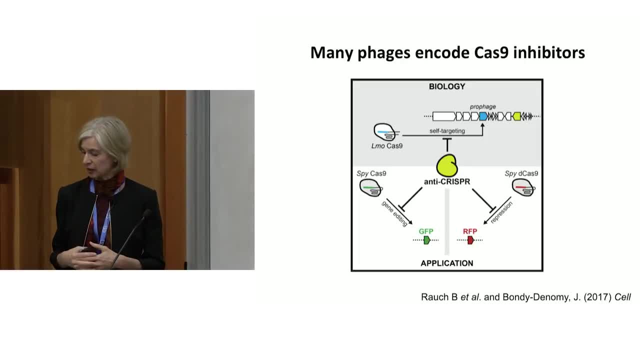 we've been very curious to understand again. how do these work and how can these proteins, which turn out to all be very small- they're typically under 100 amino acids- how do these actually operate as inhibitors and can we use? 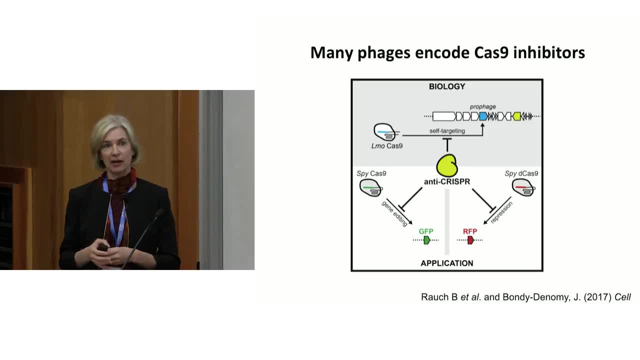 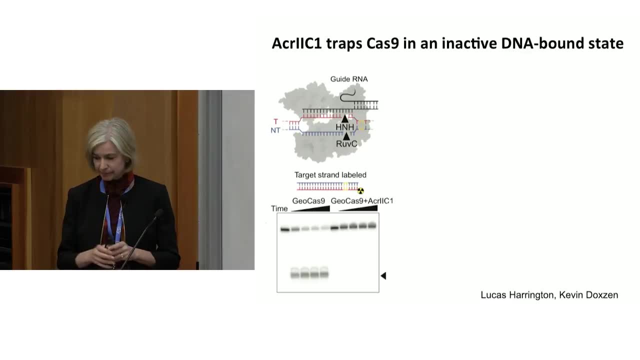 their mechanisms, to tell us more about the way that these proteins, the enzymes, actually operate. And I'm just gonna show you a little bit of data. again, this is unpublished, very new data, But one of the things that was very interesting, and this is: 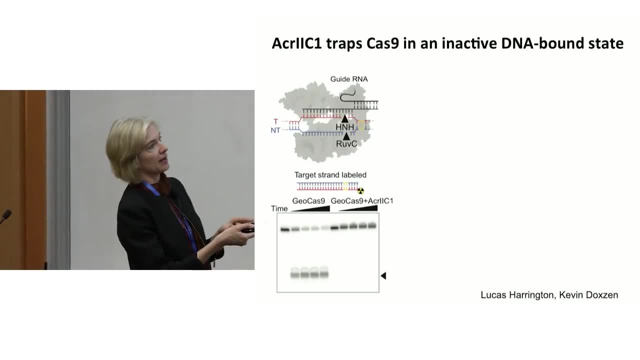 the work being done by students- Kevin Doxon, who's here and now working at the IGI, and Lucas Harrington- was they noticed that one particular anti-CRISPR protein that I'll abbreviate C1, turned out to have the ability. 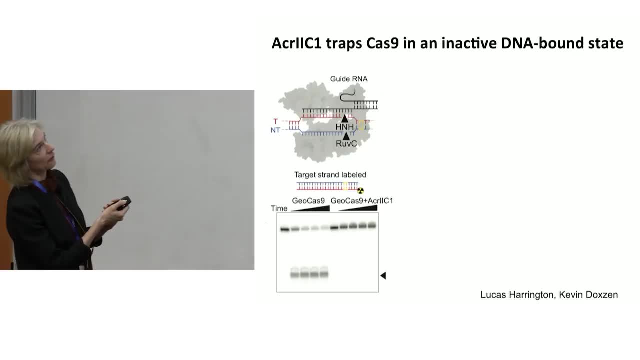 to block DNA cutting, and so what we're doing here- this biochemically- is doing an experiment where we can put a radioactive label on one end of one strand of a double-stranded DNA target sequence, and then we use this labeled DNA. 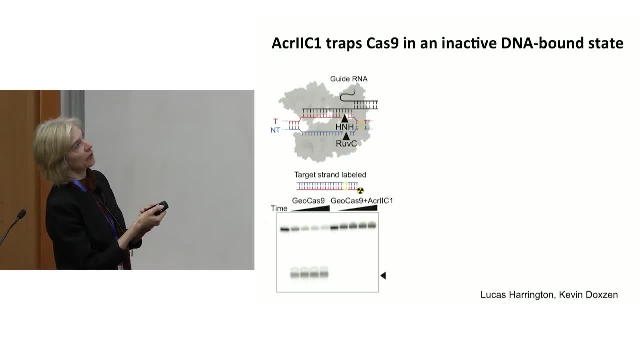 in an in vitro DNA cleavage experiment, And so if we do this with a particular Cas9 enzyme, you can see we get very nice cutting of the DNA, as you would expect if we don't have any inhibitor around. As soon as we add the inhibitor, 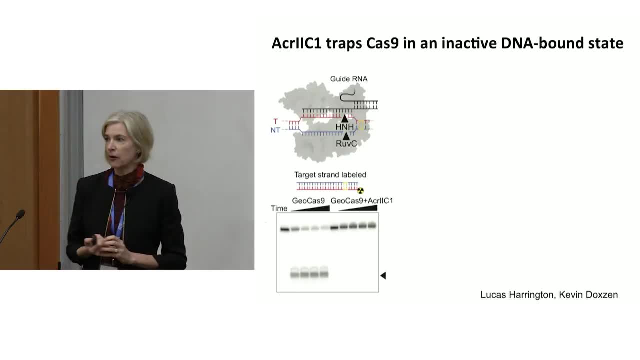 the cleavage is blocked, And so once you see that, as a biochemist you say, well, that could mean a couple of things. It could mean that this inhibitor just now doesn't let the Cas9 protein even bind to the DNA substrate. 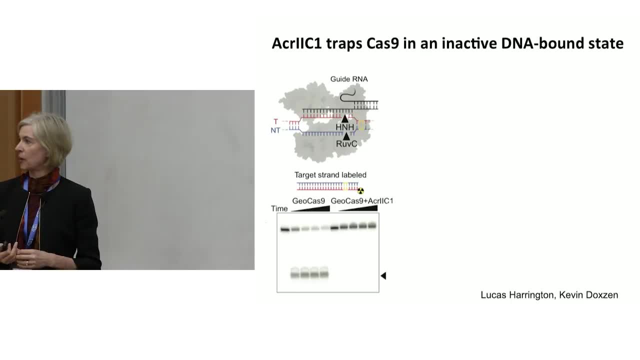 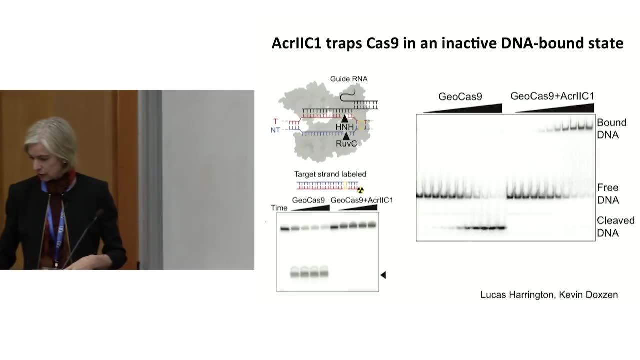 right. maybe it just prevents binding, Or it could be that it allows binding but somehow prevents DNA cutting. And so, to distinguish between those two possibilities, Kevin and Lucas did an experiment in which they used a non-denaturing gel system. So this is a gel system. 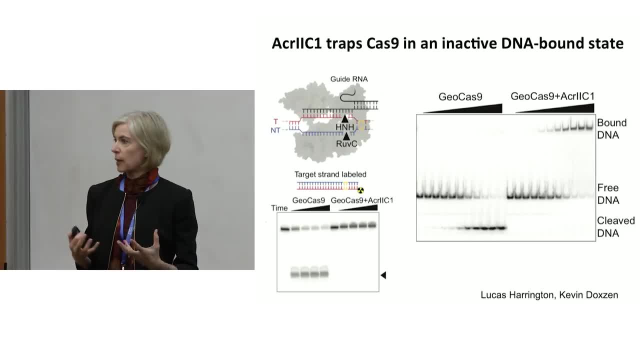 that allows us to visualize any trapping of proteins as they associate with nucleic acid. So if you look at the left-hand part of this gel system, here we're just doing, we're taking these reactions right here, no inhibitor is present and we just apply them. 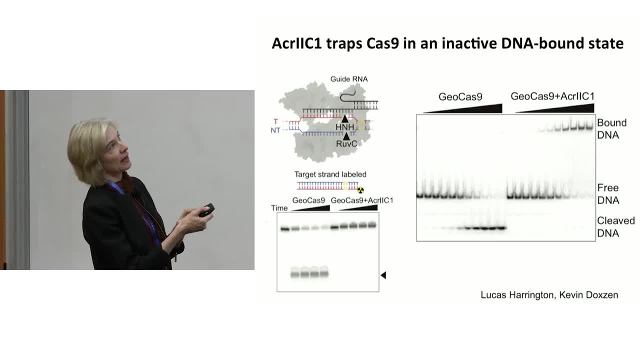 to this native gel system. So we've got our DNA is radio labeled and you can see that as we increase the amount of Cas9 and its guide RNA reaction, over time we get cutting of the DNA and the DNA dissociates. 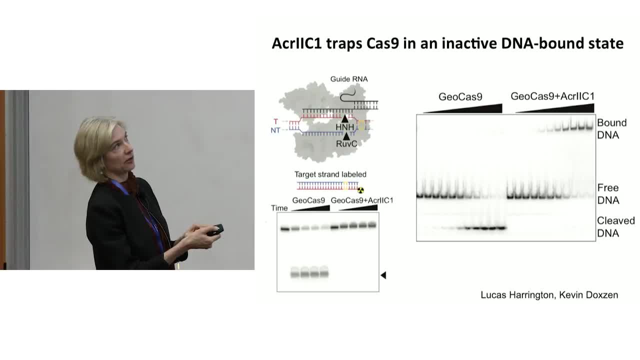 and you can see it running faster on this, migrating faster on this gel system. So that's just what you would expect to see What happens when we add the inhibitor. Very interesting result. Now, what we found was that we saw not only no cutting, 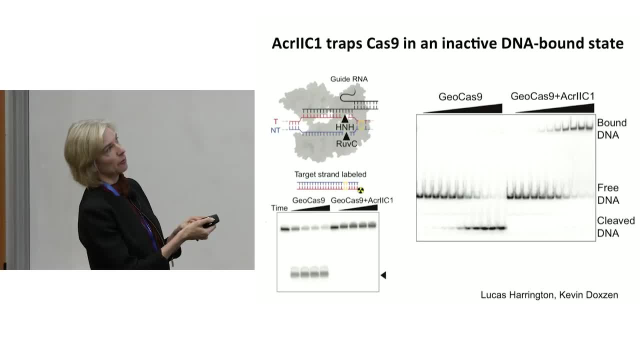 of the DNA. but we saw that this radio labeled DNA becomes trapped in a much slower migrating product and that turns out to contain the Cas9 protein and the guide RNA. So that tells us that this inhibitor doesn't prevent binding to the DNA. 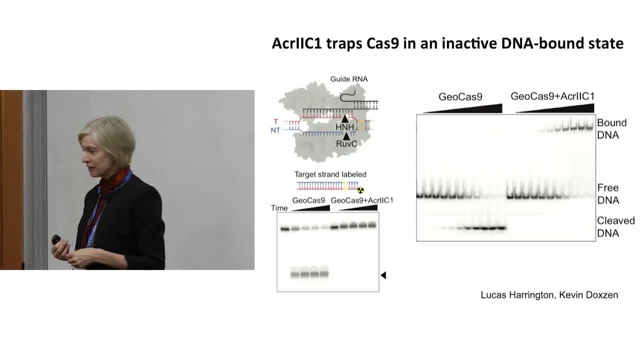 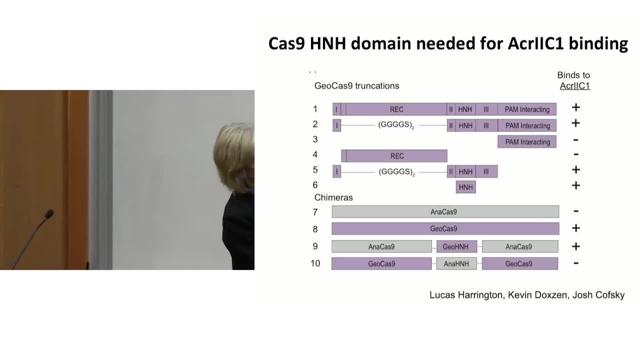 but somehow it prevents the DNA from getting cut. So it seemed very interesting: How would that work? And so, to sort that out, Kevin and Lucas and another student, Josh Kofsky, made a whole series of variants of the Cas9 protein. 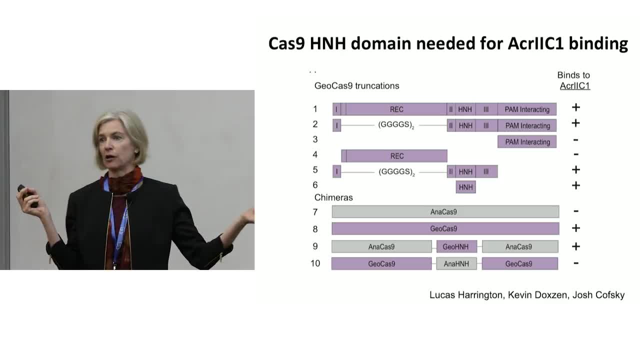 And I really just want to point out one thing: These are the ones that show kind of a linear cartoon of the Cas9 protein sequence And what we found was that in every case where the HNH domain was included in the construct, we saw that there was binding. 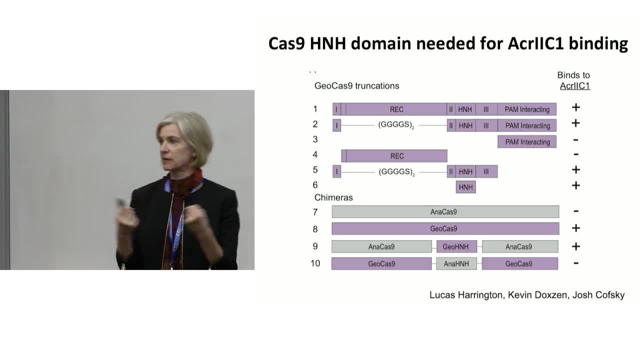 to this anti-CRISPR protein. So this is just looking at direct protein-protein interactions. But constructs that were missing the HNH domain, like this one right here, had no binding to the inhibitor, So it really looked like that was somehow the domain. 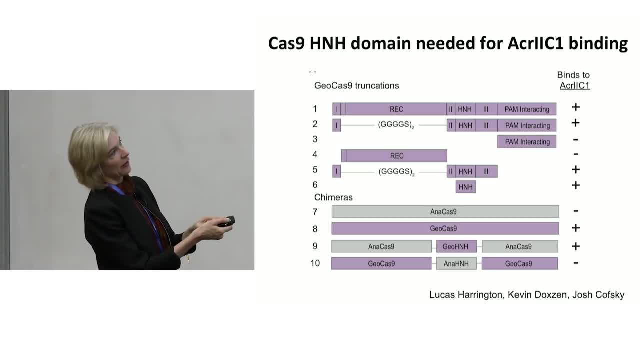 responsible for this protein-protein association And just to really bring that home, they made constructs that are shown down here, that were chimeras, in which the HNH domain from this inhibited Cas9 enzyme was swapped into a different Cas9 protein, And this now becomes capable. 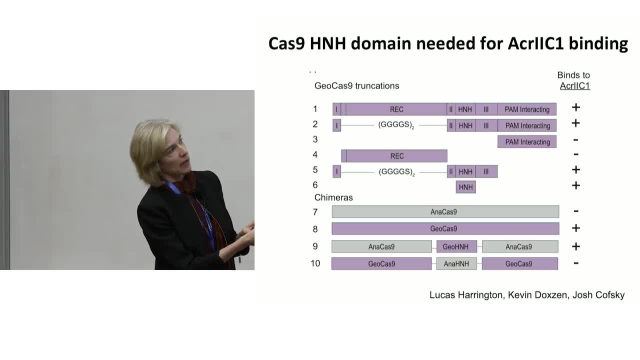 of binding the inhibitor, Whereas if we do the opposite, we use the Cas9 protein to bind the inhibitor, but we replace the HNH with a different Cas9's domain that doesn't bind the inhibitor. Now it doesn't bind anymore, So it really looks like it's specific. 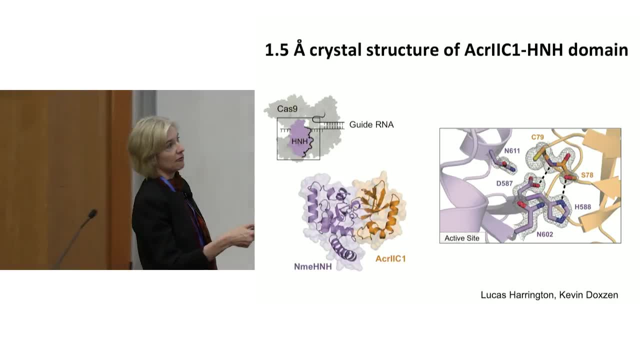 to this catalytic domain of the enzyme, And so Lucas and Kevin were able to solve a crystallographic structure of that interaction, And this turned out to show that the actual chemically important residues in this HNH domain are physically blocked by an inhibitory protein. 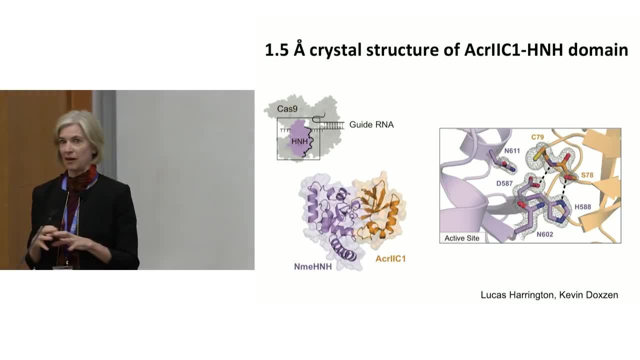 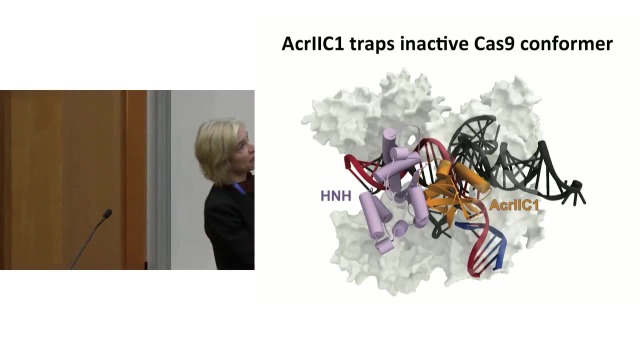 It literally grabs on to the sites important for chemistry in this domain and prevents them physically from interacting with DNA. And the way we think this actually works- and this is now a model- is that this inhibitor grabs on to the HNH domain in Cas9. 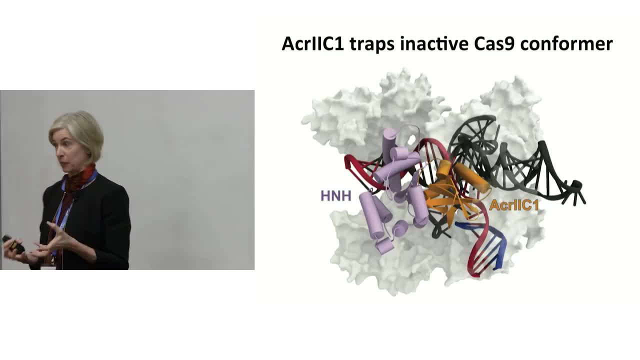 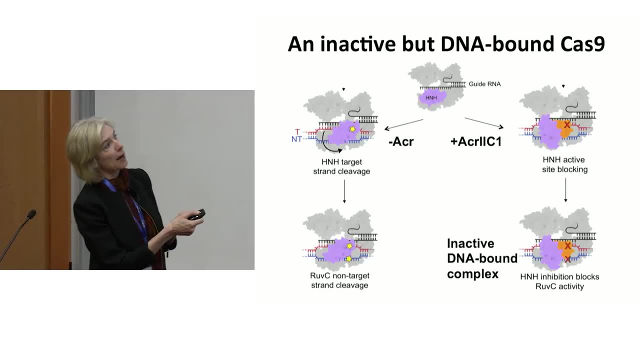 and literally prevents it from swinging into place and cutting the DNA, as I showed you that we know that there's an inhibitor that has the ability to trap the protein and its guide RNA on a DNA target, by not physically preventing it from associating, but actually just taking advantage. 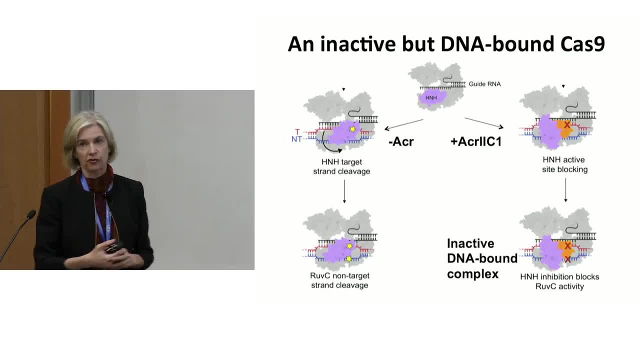 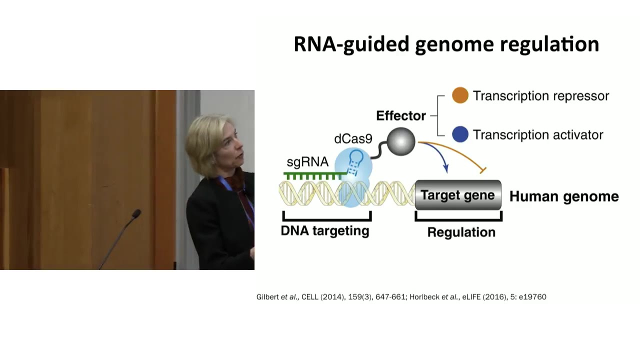 of the natural mechanism of cutting and preventing this conformational change. So kind of cool mechanism. but again, do we care about this from a technological standpoint? And I would argue that we do, and it really comes down back to the work that Luke Gilbert. 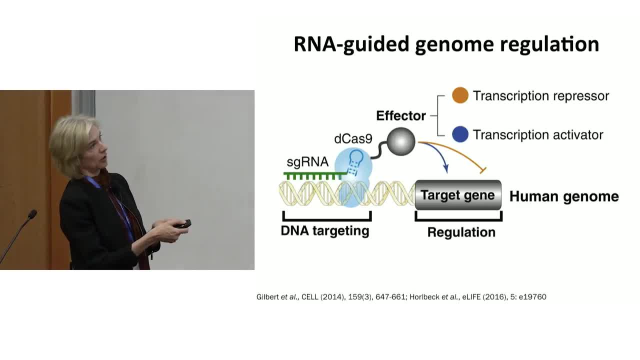 and his colleagues at UCSF have been doing, and also the work originally of Stanley Chee, who is now at Stanford, who were able to show that you could make forms of Cas9 that were inactivated by making just targeted changes to the chemically important. 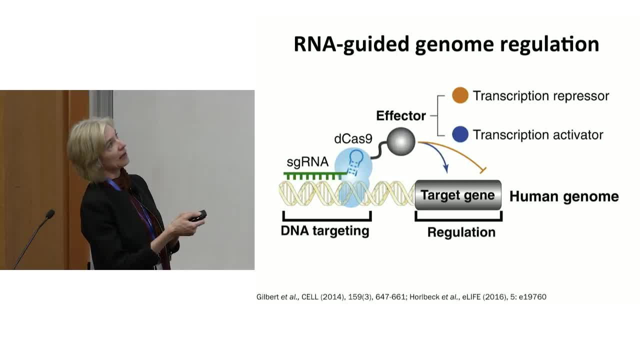 residues in the enzyme, including in this HNH domain, and then linking effector proteins to the enzyme that had the ability to repress or activate transcription. And so this shows that you know, this is sort of how one can do this kind of artificially. 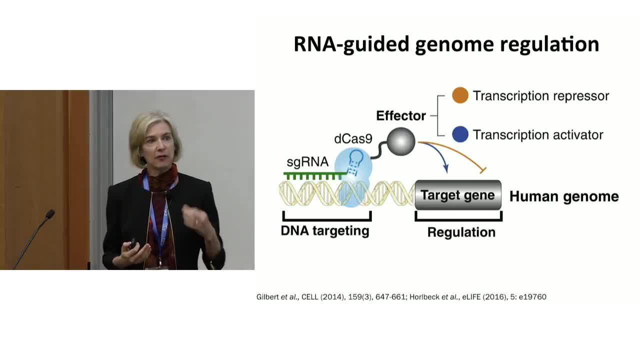 in the laboratory. but what if it's true that? what if it turns out to be the case that in phage or bacteria that have this particular anti-CRISPR protein, they can actually block DNA cutting by Cas9 and thereby allow it? 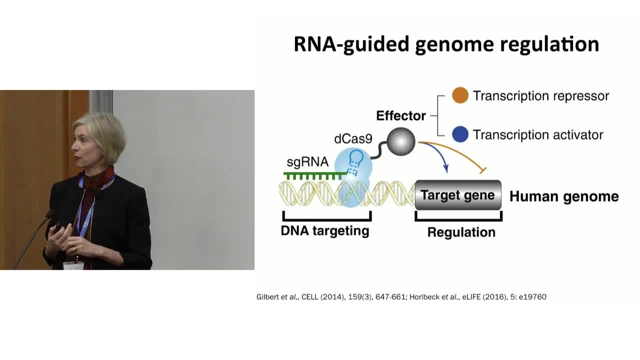 to function in a regulatory fashion. so that's something that we're now testing. So it may be that this really kind of allows phage or bacteria to expand the function of Cas9 naturally in cells, not by making mutations in the enzyme, but simply by blocking its ability. 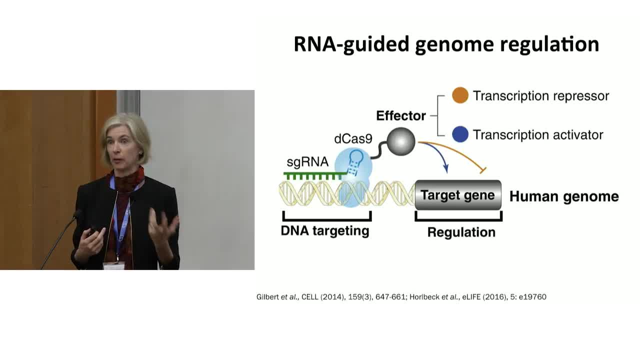 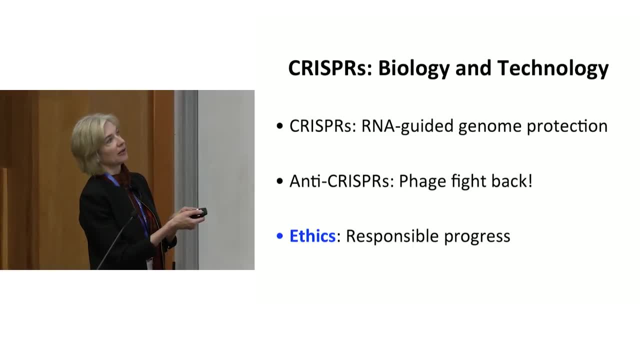 to cut DNA but retain its ability to bind in an RNA-guided fashion. Okay, so just in the last minute or two here, I just want to say a little bit about what I call responsible progress, And so you know one of the things. 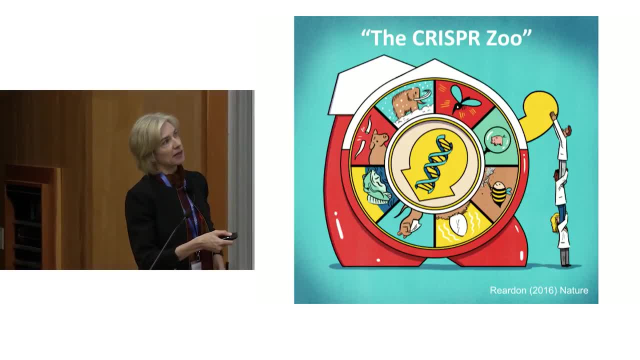 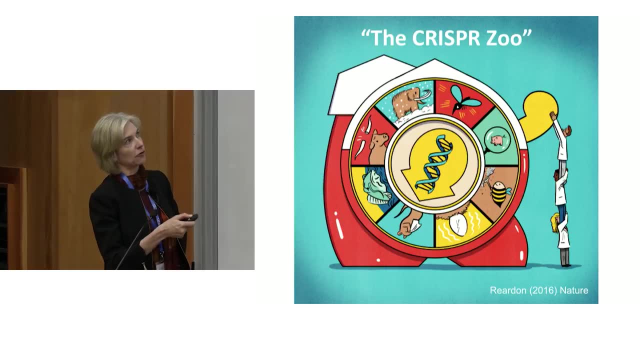 that's been really exciting over the last few years is just the rapid adoption of the Cas9 technology for all sorts of gene editing applications, And this was a cartoon that was published in Nature last year just showing that, as Dana said, now there are over 100 organisms. 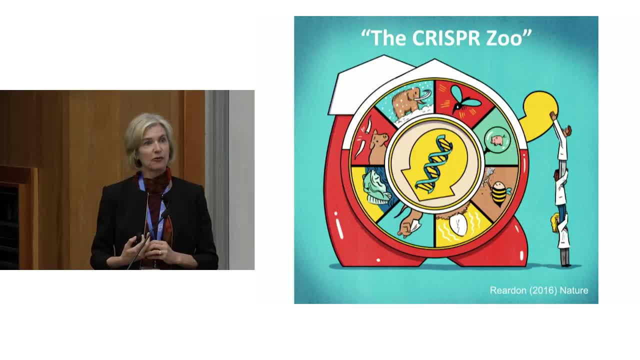 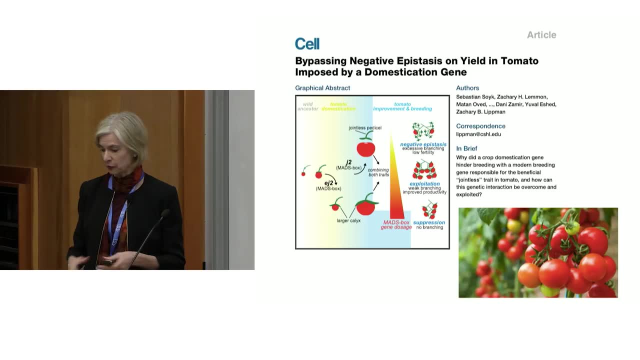 and cell types, many, many more cell types that have been modified using this system. And just to show you some of the very recent things that have been happening- and this is actually on the cover of the journal Cell recently, where a group at Cold Spring Harbor 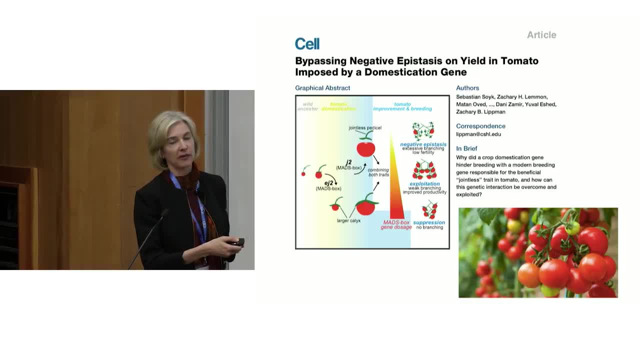 was able to use the Cas9 system to make targeted changes in tomatoes, And they were doing this to actually separate two genetic changes in these plants that had been selected by traditional plant breeding but couldn't be separated by traditional plant breeding because of the length of time. 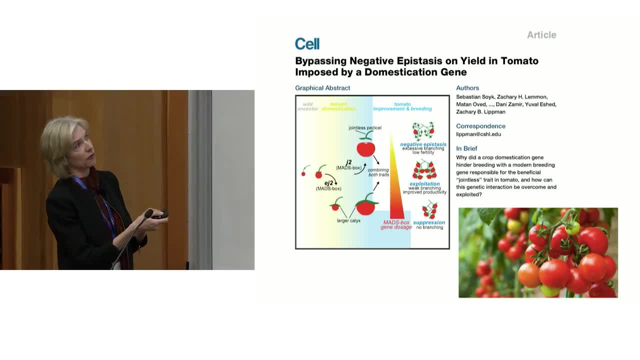 it would take to actually do that. They were able to knock out a number of genes and thereby create plants that have much stronger branches. They were able to hold heavy fruit loads. like this very practical use of gene editing and doing something that would have been difficult. 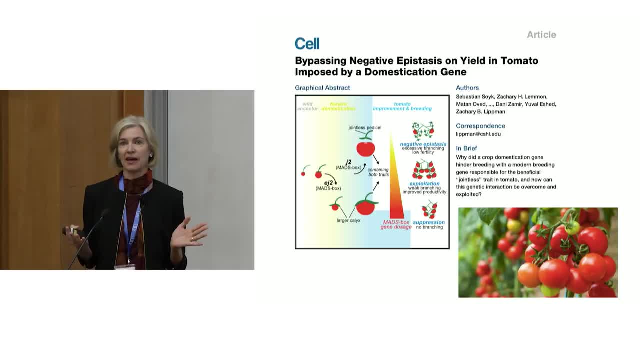 if not impossible to do with traditional methods. Why was this on the cover of Cell? Well, I think it's just sort of a harbinger of where this is all going, that in the future people are going to be able to do things in crops. 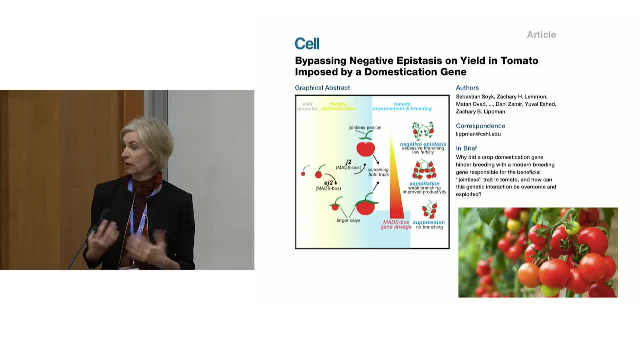 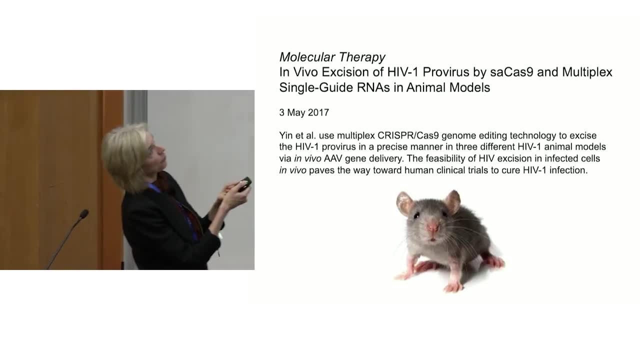 but also in plants that people are growing in their gardens, and to do things that will create traits that are very useful in different ways. Another recent example was this one right here. So this was a Chinese group that published work showing that you could actually cut out. 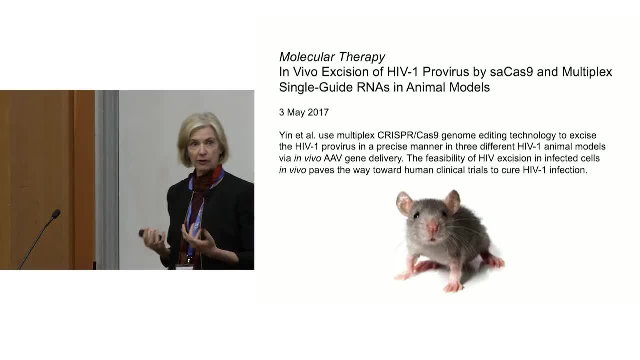 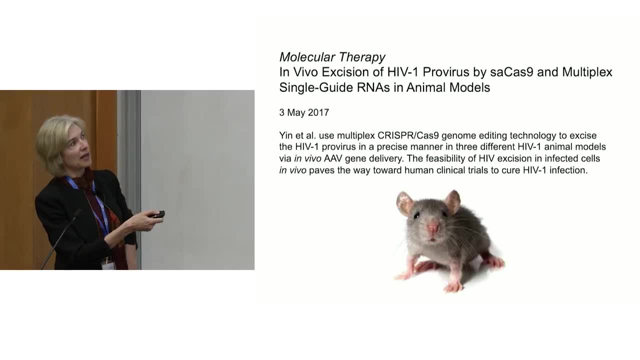 integrated HIV pro-viruses from the genomes of mice and thereby effectively sort of cure, if this is actually operating in nature, except here we're doing it in mice Now. will this be an actual therapy for HIV? Probably not right, Because it might be very hard. 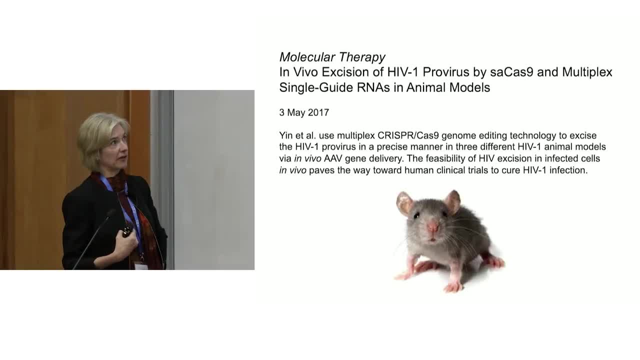 to actually cut all the pro-viruses out of infected cells in these animals. On the other hand, it shows the precision of the technology and it also points to the fact that there's a lot of interest in using this system to protect organisms from viruses. 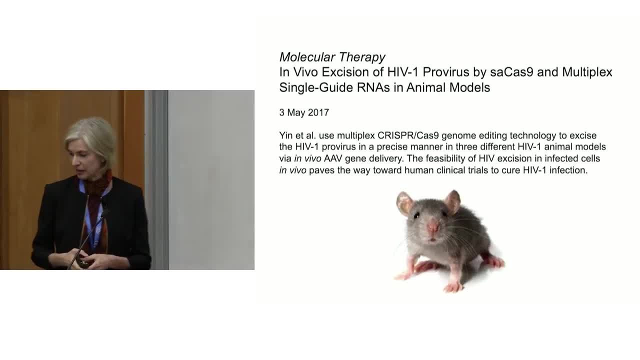 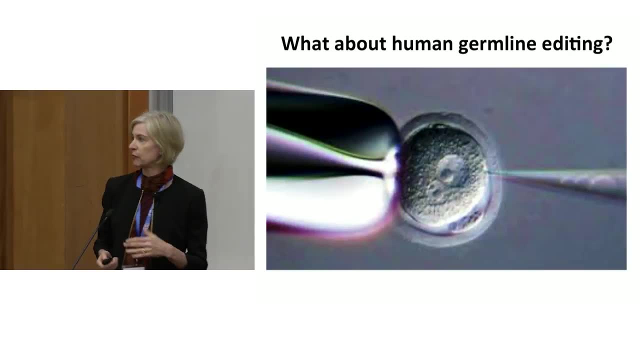 by harnessing these activities in ways that are analogous to what we're doing here. And finally, then there's germline editing, right. So all of the editing that's being done at the moment for clinical use is being done in somatic cells. 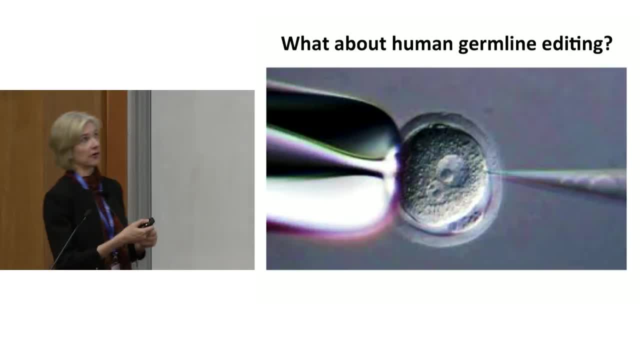 in cells that are fully differentiated, But we know that this technology works very nicely also in stem cells. It works in germline cells. This is an example from Russell Vance's lab here at Berkeley showing a fertilized mouse egg held by a pipette. 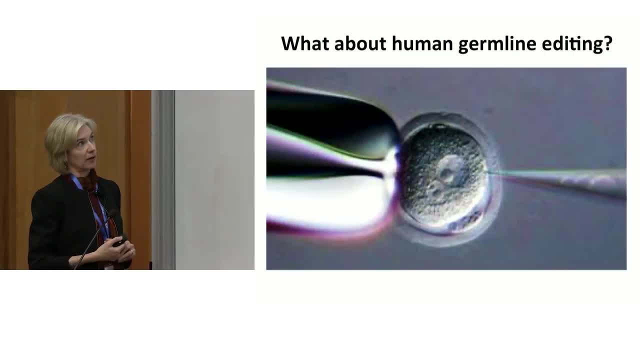 and we're seeing a needle coming in into this very early embryo. And when those edits are made to the DNA they become heritable right, They become part of the entire animal, including its germ cells, so they can be passed on. 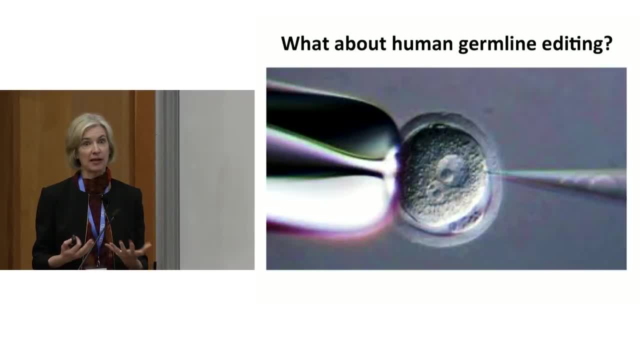 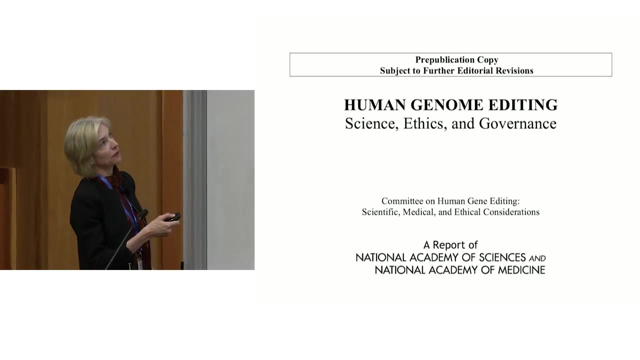 to future generations, And if that's done in a human being, then we have a situation where we're making changes that become embedded in human populations in principle, And so this has triggered a lot of discussion around the world and has led to the release very recently. 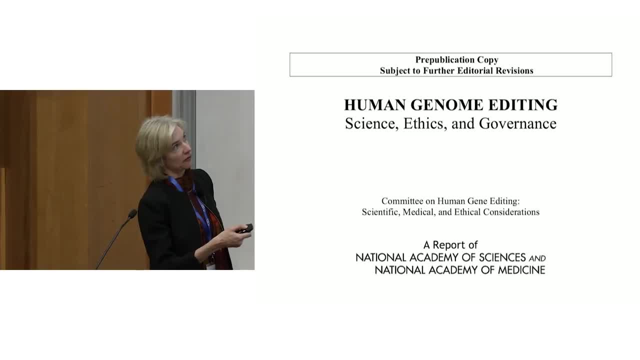 of this document here by the National Academy of Sciences on human genome editing which, if anyone's interested, you can download it and it really goes through all of the implications of this, especially for human germline editing and sort of a roadmap. 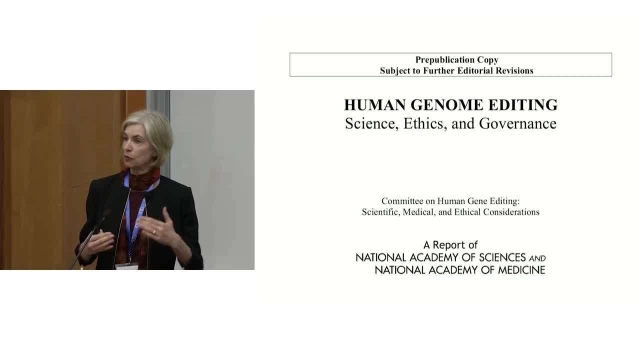 for how we as a scientific community, global community, can move ahead to ensure that there's robust research going on, but that it's not sort of impeded, but that we also have appropriate regulations around this kind of very powerful sort of application. 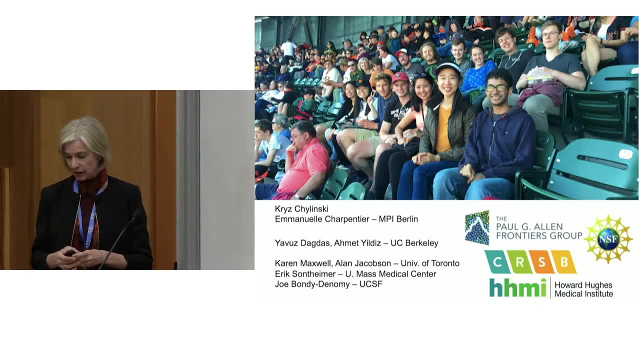 And you'll hear more about that later this week. as Dana said- And I'm gonna close just by mentioning that all of this research is done, of course, by students and postdocs in various laboratories, including our own, but we've had many, many 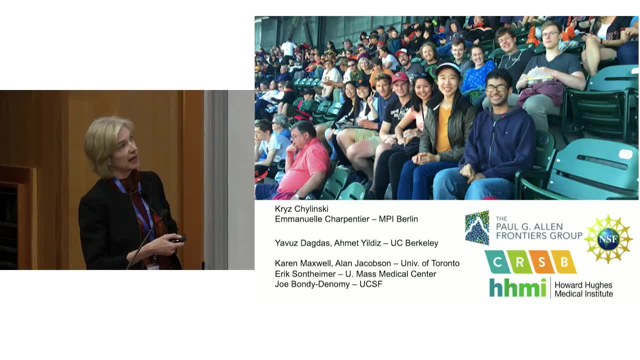 many wonderful collaborations, and I'm just mentioning a few of them here. These are some that I mentioned today. The University of Toronto are actively working on anti-CRISPRs and we've had a great time collaborating with them, as well as with Eric Sondheimer. 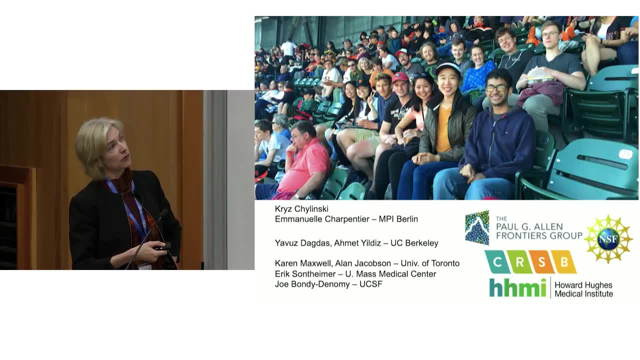 at University of Massachusetts And I mentioned these folks. Science can't be done without funding and I think we all have to be aware that right now we're facing a very difficult situation, especially here in the United States, where there's an active push. 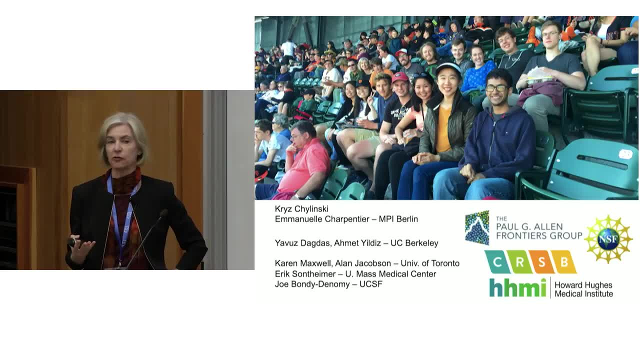 by our federal government to cut back on research funding, which is the kind of fundamental research that I talked about today, And so you can see that if we really do that, I think we're gonna put the US at a severe disadvantage in terms of discovering new technologies. 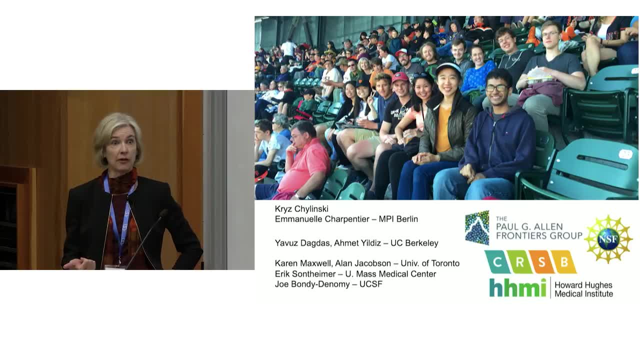 and moving ahead in the areas of research that we know are gonna be important not only for human health and our environment, but also for stimulating the economy, creating jobs, et cetera. So I would ask all of you to think about ways that you can communicate the importance. 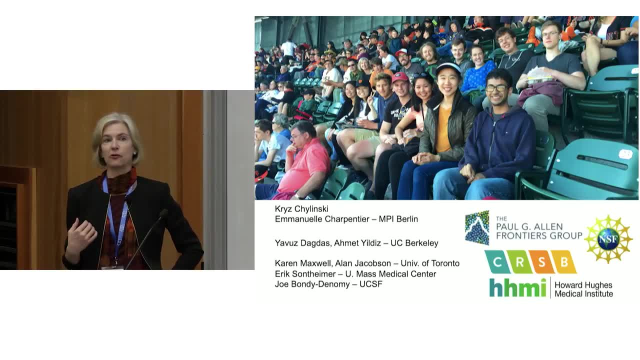 of the science that you're doing, where all of us are taxpayers- to take appropriate measures as they feel so moved to support science funding at a fundamental level, And I'm gonna stop there- I don't know if we have time for questions. 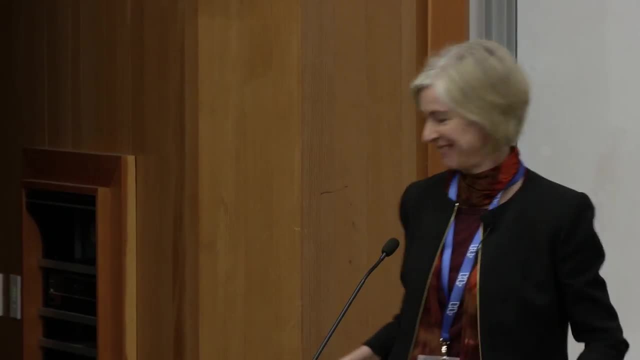 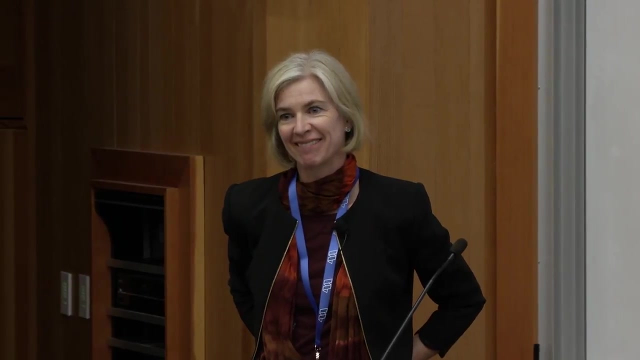 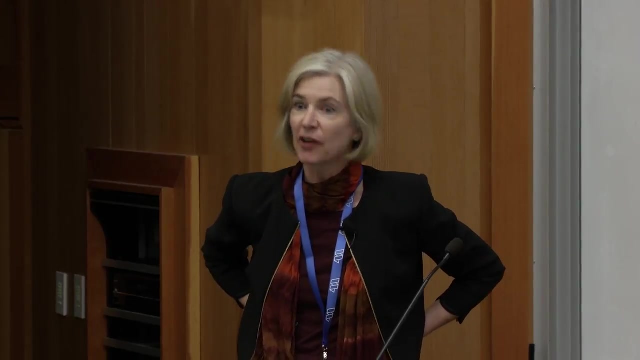 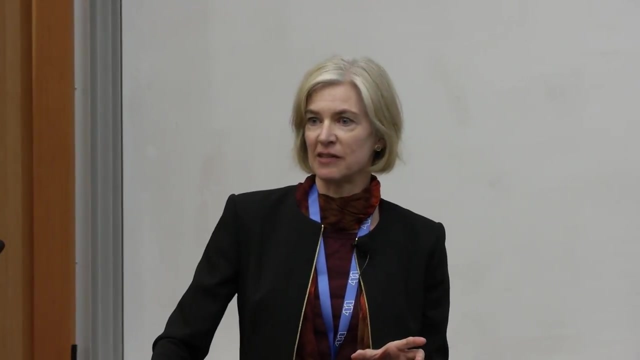 but if you have any, I'd be happy to try to answer them. Yeah, Yeah It does. It hangs onto the DNA. Yep, I didn't have time to say that, but that's right. It has a very high binding affinity. 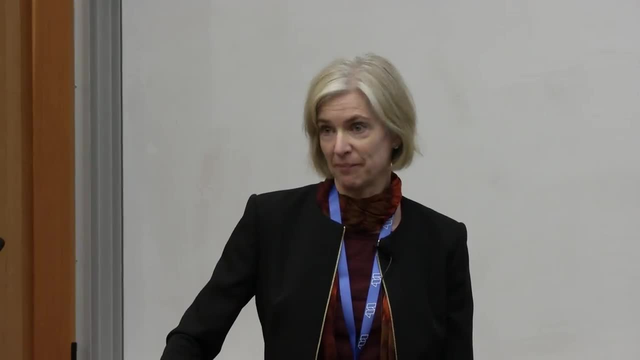 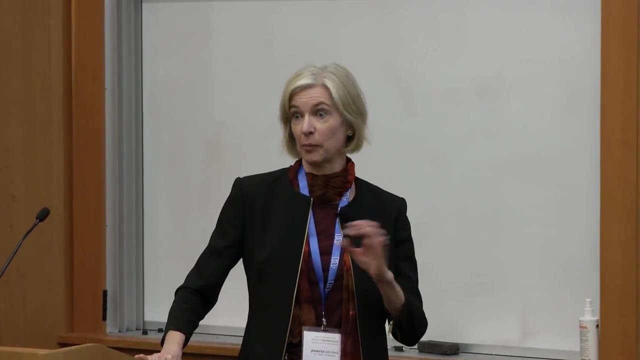 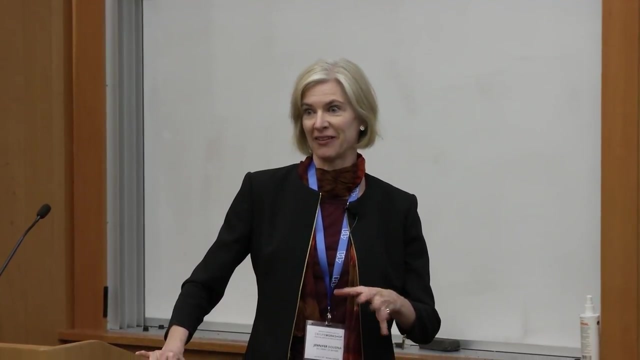 to the DNA, even after cutting. Yes, Yep, yep, You can do that Actually using this FRET assay. we can do that, Yeah, yeah. So there's a lot of nice in vitro. of course, We're not doing it in the context of chromatin. 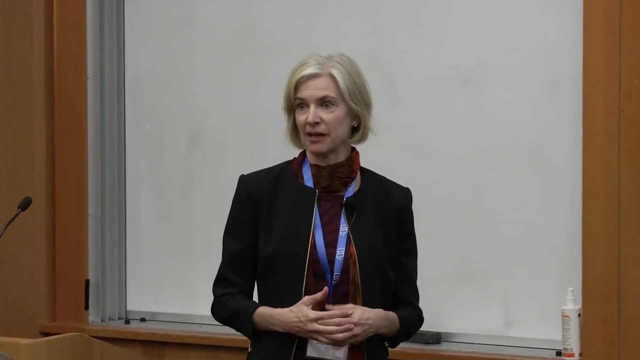 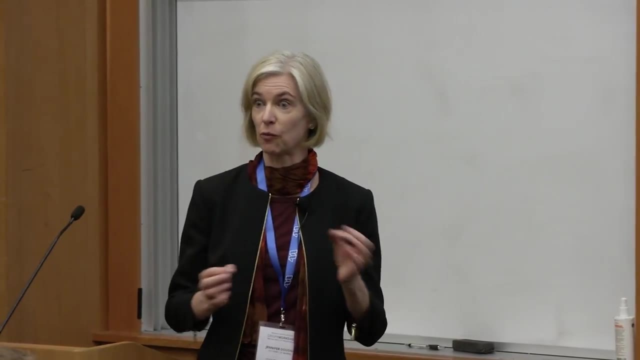 So then we have to have other ways that we can try to relate those measurements to what might be happening in cells, And there are already. we've done some of this and there are other labs looking at in vivo imaging of Cas9, so you can really watch behaviors. 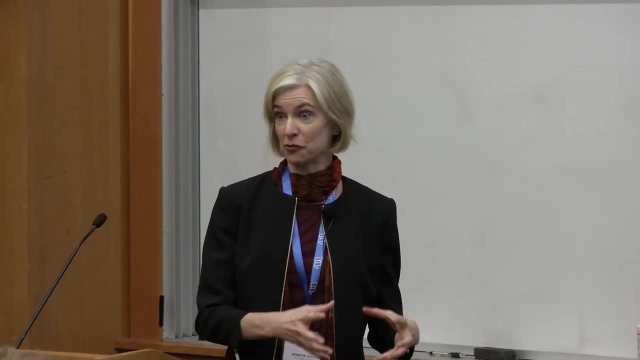 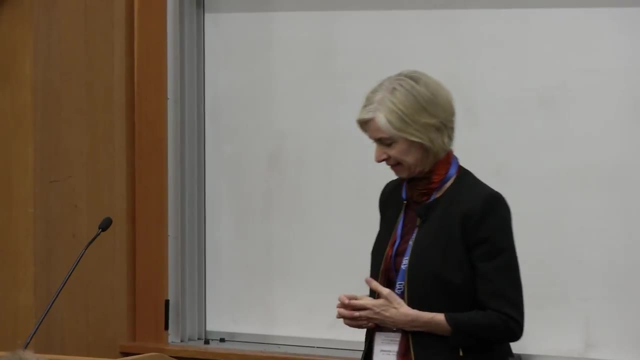 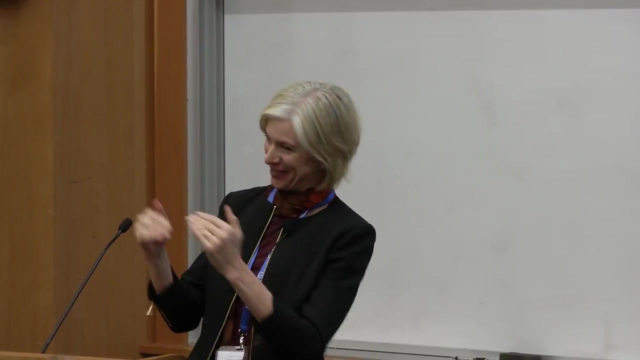 in the nucleus as well. So I think over time we'll build up this very nice continuum between biochemical experiments in vitro and in vitro. Yeah, Other implications of the existence of anti-anti-CRISPR proteins You can imagine there's probably. yeah. 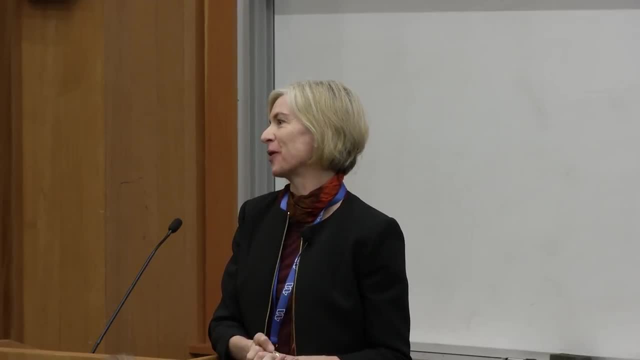 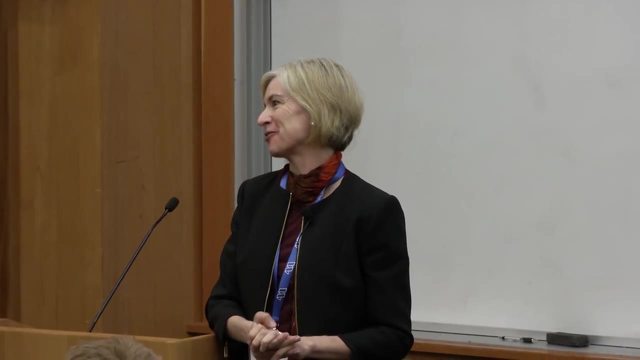 anti-anti-CRISPRs and yeah, Sure, I mean I think it's sort of one of those things where, if you can imagine it, it's probably out there somewhere in biology, And if it's not, out there already, 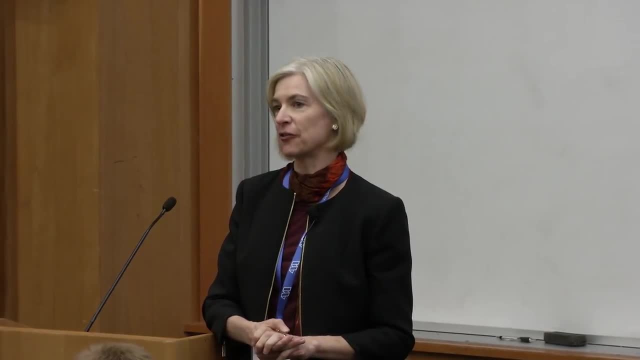 you can imagine ways that you could potentially engineer such things right. So I think one of the things that's going on right now is the movement towards using engineered proteins or natural ones to control the activities of Cas9 enzymes in cells for the purpose of safety. 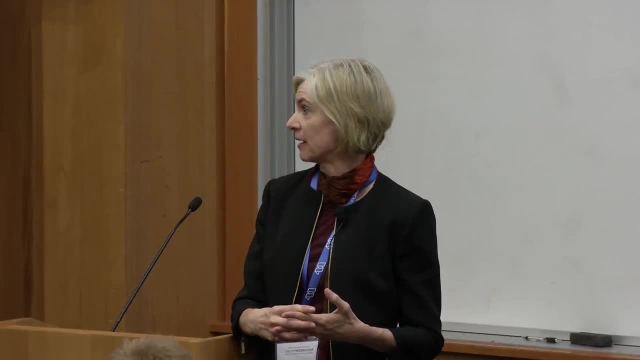 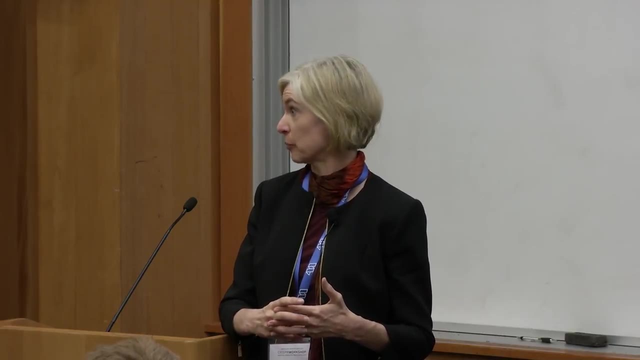 and also for the purposes of accuracy, And in fact I think he just stepped out, but his group with us have recently been using anti-CRISPRs for that purpose right, Where you can actually limit activity in cells and reduce the activities. 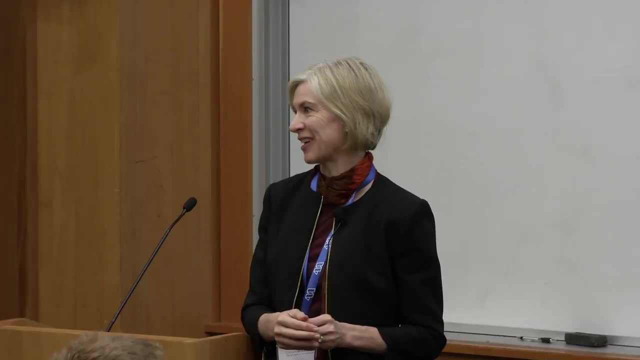 that might be occurring at off-target sites. So I think you know this is sort of an exciting time where we're seeing very rapid technology development around not the fundamental core activity of Cas9, but really how we modulate that activity in cells. 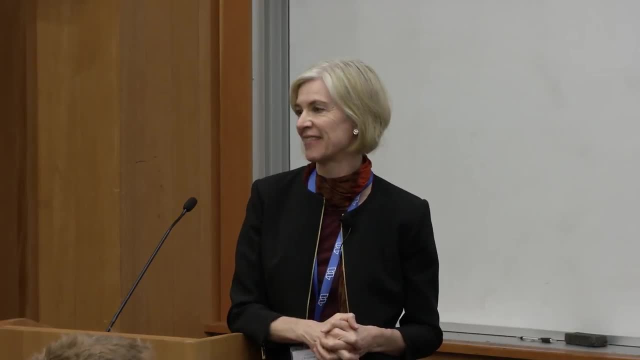 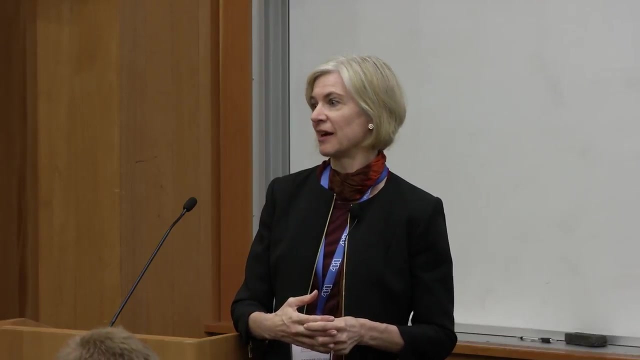 using some of these types of approaches? Yeah, How does adaptation work when the vacuum gets pumped? Yeah, that's a great question. So there's a lot of work going on on adaptation. so that means basically we have two viral sequences into these CRISPR arrays. 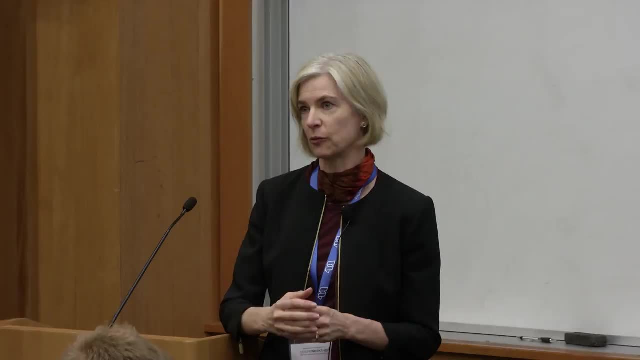 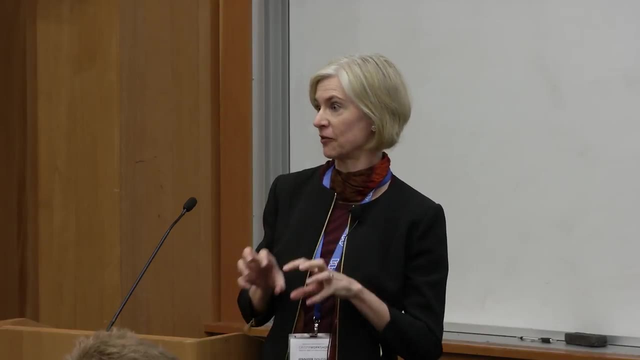 And I didn't have time to tell you about it. Our lab has done a lot on this and there's other labs, of course, contributing as well, but we know that there's a particular CRISPR integrase. It's a two-protein complex.